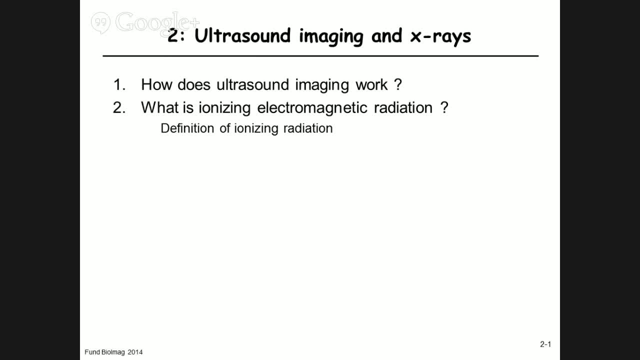 Then we're going to ask the question: what is ionizing radiation? And lastly, we're going to finish today with the question on how are X-rays produced, Because obviously the naturally occurring radioactivity levels are not sufficient to do imaging. 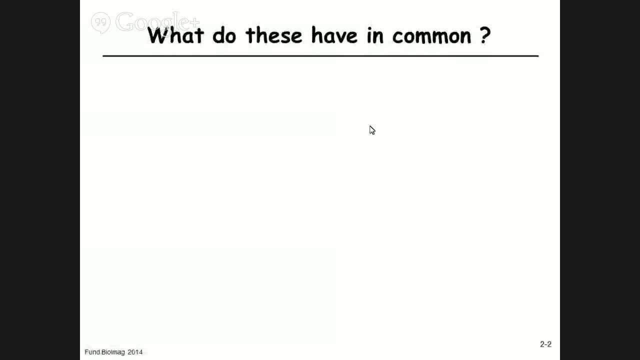 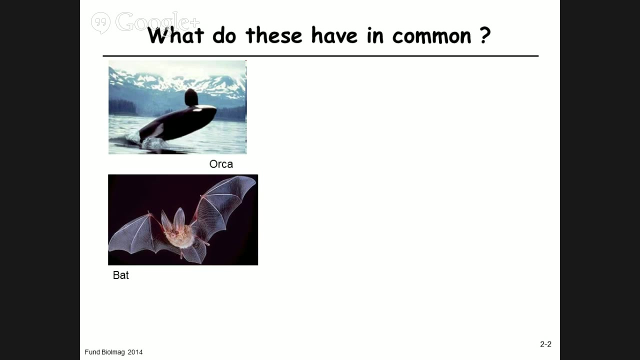 OK, so let's look at some images here, And the question is: what do they have in common? We've got the orca- I think you all recognize this animal. We have the bat. We have the ultrasound scanner. We have boats. 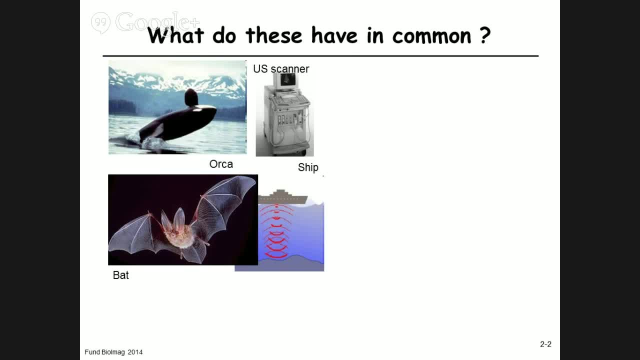 So what do they have in common? OK, They use ultrasound for location. Yes, so does the bat, So does the ultrasound scanner and the boat Radar. What does it have in common with the above four? Well, radar localizes. 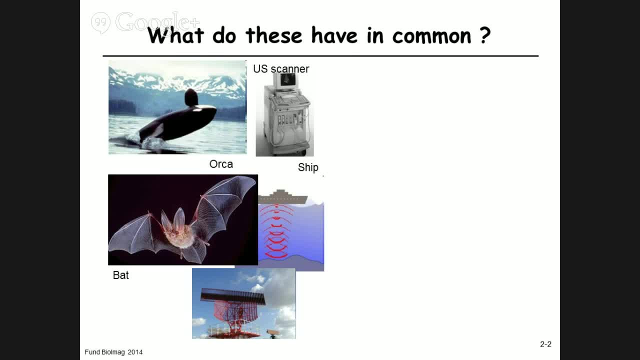 It's an incoming airplane with radar, so it's not ultrasound, But the principle of localization is the same, So it's a way of imaging, if you will. So briefly, the ultrasound transducer is a device like this. It's got some backing material, electrodes. 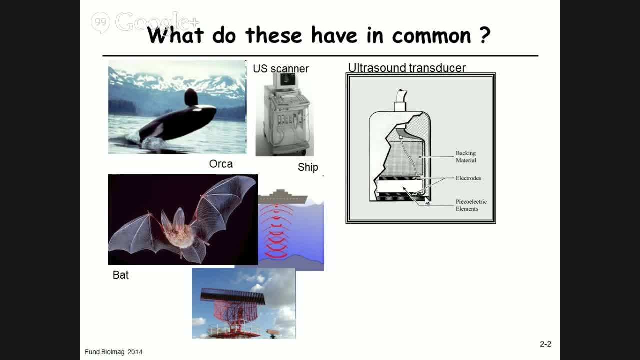 some piezoelectric elements. I won't go into too much details, It's just a small device. This is the scan head And this is for science. It's a precise comparison. Here's the single crystal of the scan head. 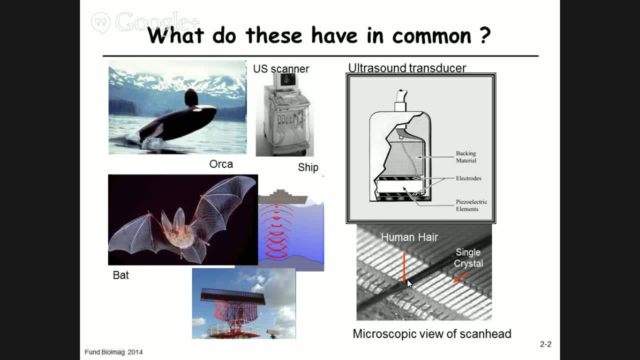 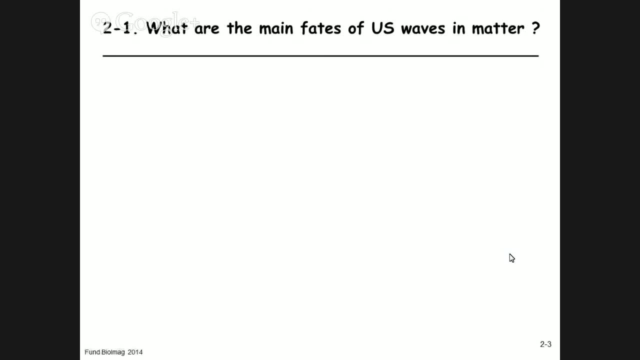 It's a transducer and receiver as well, And this structure here is a human hair, just to give you an idea how small these elements are. So let's look at the fates of ultrasound waves in matter. What are the principal fates that ultrasound? 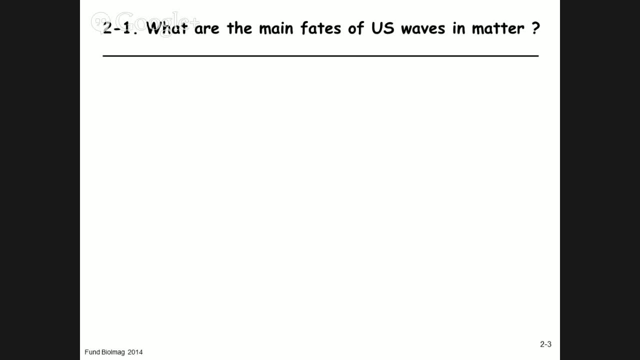 can undergo in living tissue. We're focusing here on living tissue, of course. So, number one, we have attenuation. If you have matter. the ultrasound or the sound waves will not just go on forever. I think that's the principle of soundproofing. 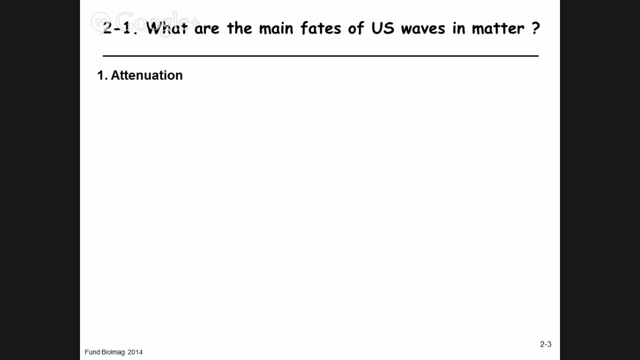 That's the principle of your apartment, so you don't hear too much what's going on in a neighbor's apartment or your roommate next door. So the sound wave travels through the substance, but it loses energy as a function of space. So here's my opposite. 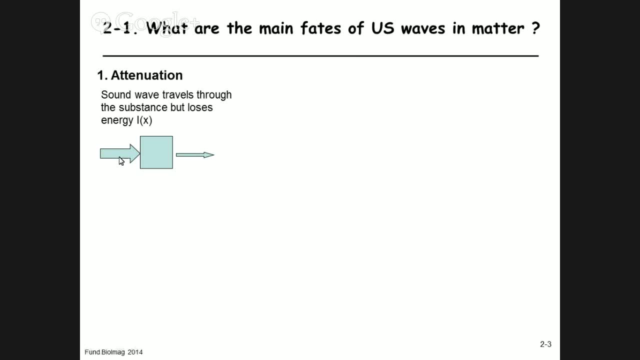 Here's my object, Here's the sound wave going in. It has a certain intensity And once it's passed through the object it has lost in intensity. And that is described by a simple exponential law with some factors to consider in the exponent. 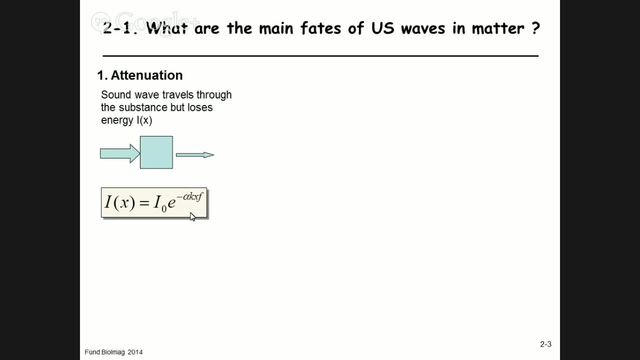 So we have the initial intensity and then, as a function for a homogeneous object, as a function of space, this intensity decreases exponentially. So what are these factors that we have there? in the exponent, We have the attenuation coefficient alpha, which is given in decibels per centimeter per megahertz. 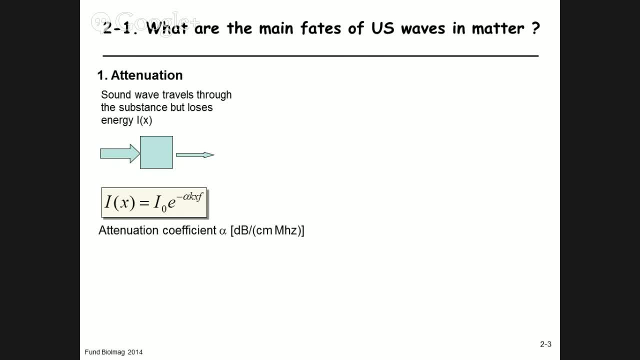 So decibels per centimeter makes sense. It's the attenuation per centimeter For units. we need that. And then it's per megahertz because it is frequency dependent. Usually it's given in the units of decibel. 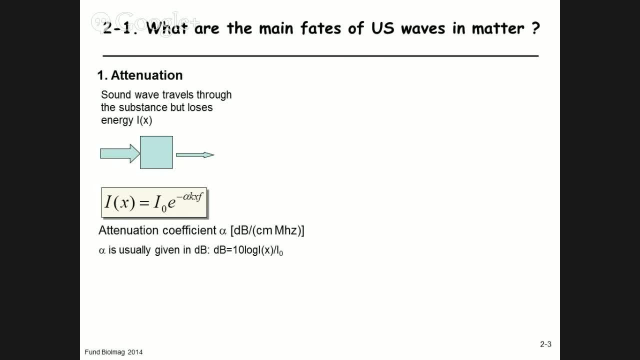 And the decibel here for energy is 10 times the logarithm of the rate. That's an issue of the intensity divided by the original intensity. So what does this mean? For physicists, decibel is a horrible unit, For engineers less so. 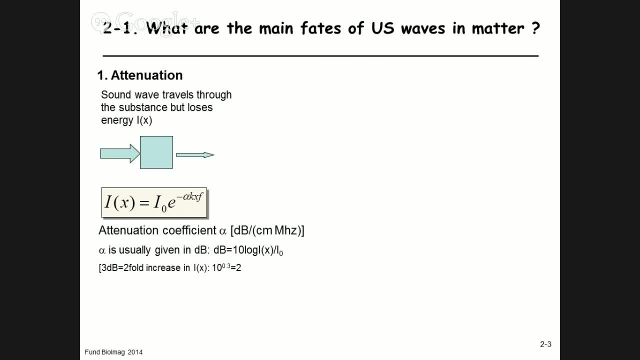 Much of engineering is done And I always have difficulty figuring out what is decibel, so I wrote it here. So three decibels corresponds to a two-fold attenuation. That's easy to remember. Six decibels is four-fold, et cetera, et cetera. 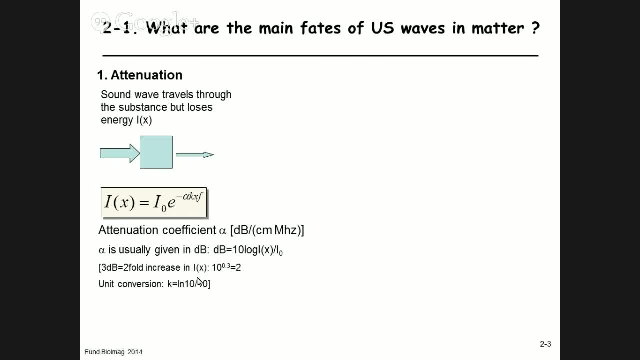 Just to give you an idea what this means. Then we have a unit conversion factor, So we have alpha, We have unit conversion factor k. That's logarithm, natural logarithm of 10 divided by 10.. That's just that the equation works. 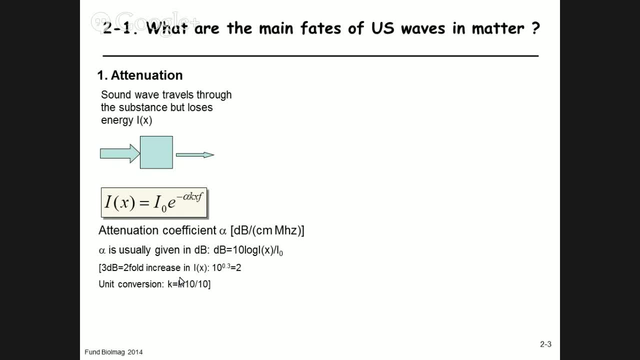 between the unit of decibel and this exponential law. So typically what one has is about a half a decibel per centimeter, per megahertz, And of course f- here is the frequency. I forgot to mention that. So we have the attenuation coefficient conversion factor. 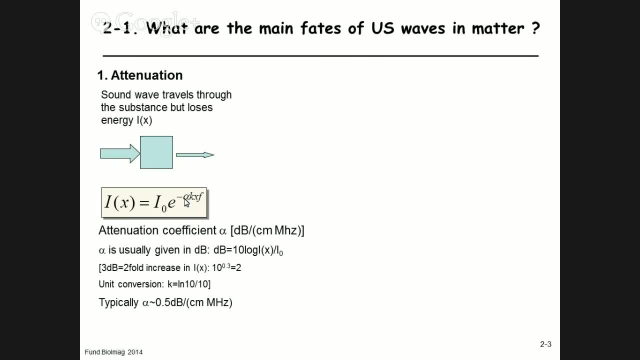 the position and the frequency. So in units this gives us something per frequency times frequency. So it's attenuation per centimeter times centimeter. This has to be without units, so that works quite nicely. So what does an attenuation coefficient of a half a dB per centimeter per megahertz mean? 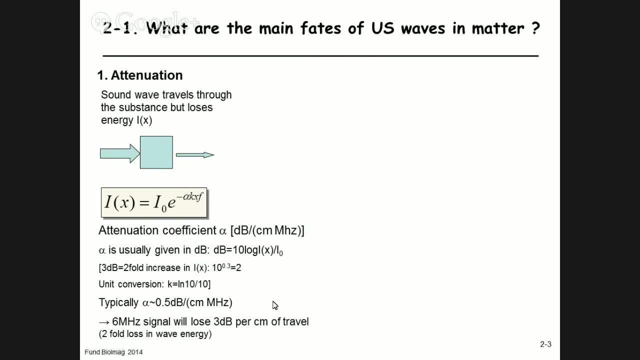 I'll give you an example now. It means that a 6 megahertz signal will lose 3 dB of intensity per centimeter of travel, So that's a twofold loss in wave energy. That's what this roughly means. OK, so that's the first fate. 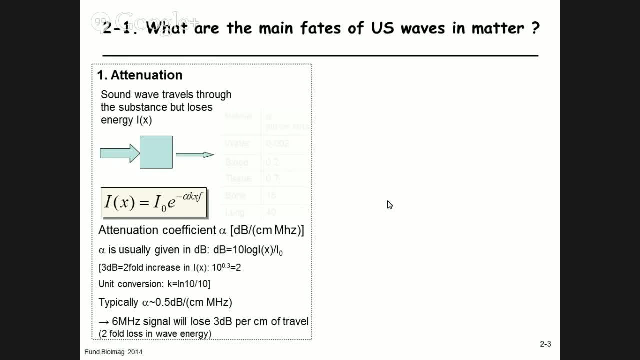 The ultrasound waves are attenuated in the tissue. So here are some attenuation coefficients for different materials. So water, it's very weak, Hence the orca, hence the boat. OK, In blood it's a bit stronger: Tissue 0.7 in this example. 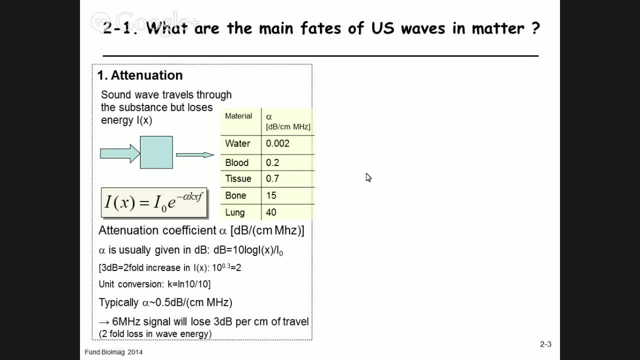 Bone much higher And in the lung it's 40,, so very high attenuation. The second fate is refraction. So refraction means if the sound wave hits an interface that's oblique, it's deviated. Now what does it mean: hit an interface? 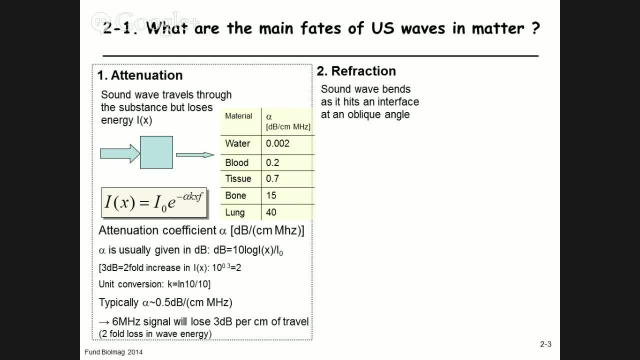 You can just think of normal sound. You've got a wall, You talk to the wall. Your sound wave is going to be reflected. A good concert hall has very good sound properties. It's very well constructed so that the sound from the orchestra is very well represented with the audience. 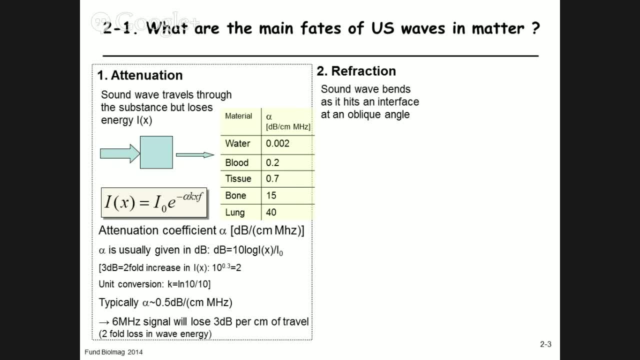 Same one would hope here for the lecture hall, But as I'm speaking here, the sound from the speakers is also being refracted by all the different surfaces. So here's the incoming wave, and then it is deviated because it hits it at an oblique angle. 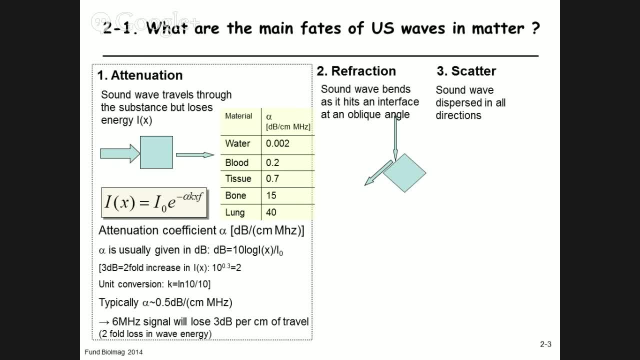 The third fate that I'm going to mention now: the refraction. we're not going to deal with it too much, I'm just mentioning it here for completeness sake. so we have covered the main fates of ultrasound. What is scatter? 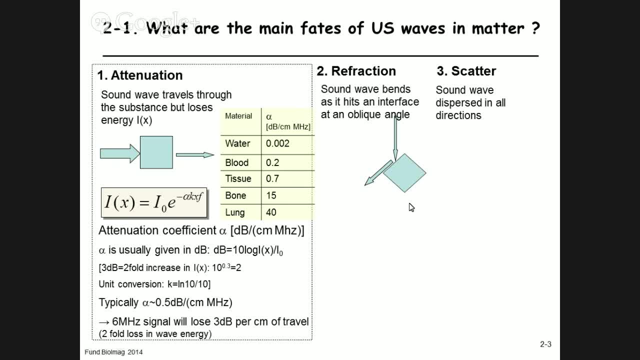 Scatter means the sound wave is dispersed in all directions. So here's an example, here's my object: The sound wave hits it and then it's split up in all sorts of directions and scattered, therefore scatter. Okay, so we've got three. 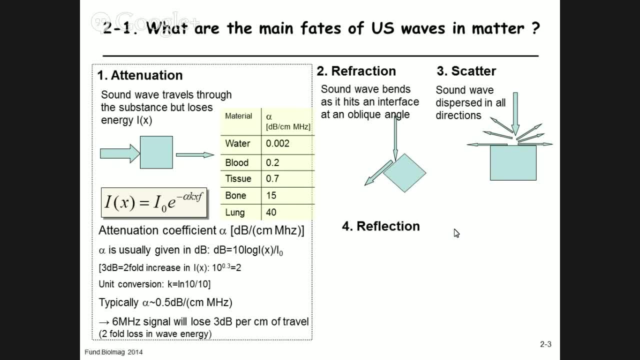 Interactions. and the fourth one is reflection, So the sound wave bounces back to the observer, or to the probe in the case of imaging. So here's again my object: Sound wave comes in and it's bounced back. Okay, you've all actually pretty much used this before. 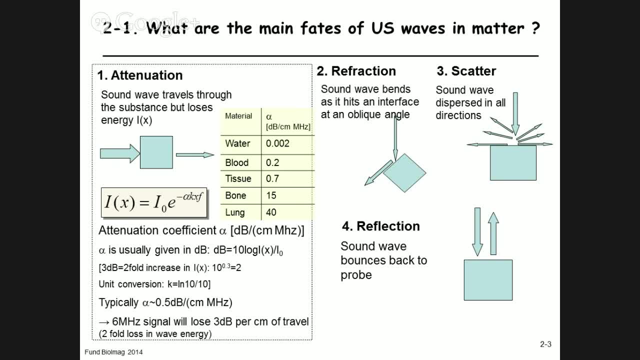 Ever remember the moment you're somewhere in a tunnel and you holler and it comes back to you. Done that, No. In the mountains, sometimes in front of a big vertical wall, you holler and then it comes back to you. 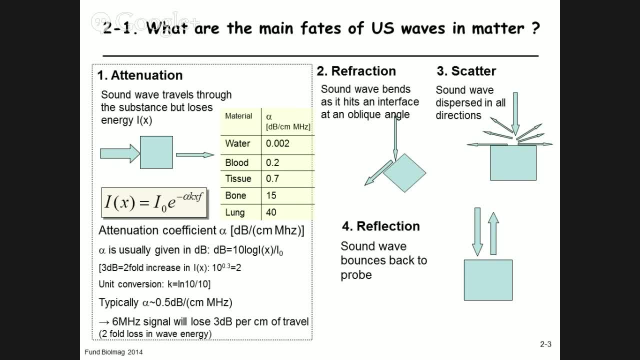 That is reflection. Okay, now in soft tissue we're going to have a similar situation. That's an extreme case. the interface air to mountain, for example, or in the tunnel, And reflection is the key mechanism by which ultrasound is used to image the tissue. 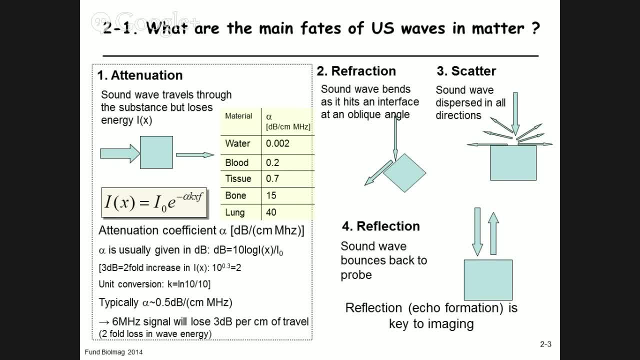 That's the effect that we want. That's the effect that one uses to produce images. Refraction scepter produces distorted images or, worse, noisy images. And attenuation weakens the signal and also produces noisy images. So that's actually the unwanted part. 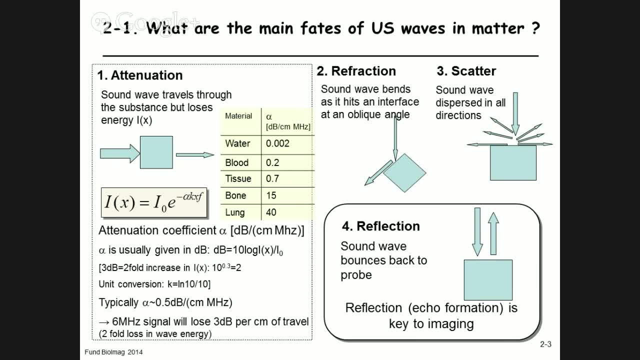 What we really would want is a situation where we would have tissue, where there's no refraction, there's no scepter, no attenuation, just reflection. That would be ideal. Ideal doesn't exist, so we have to leave with the others. 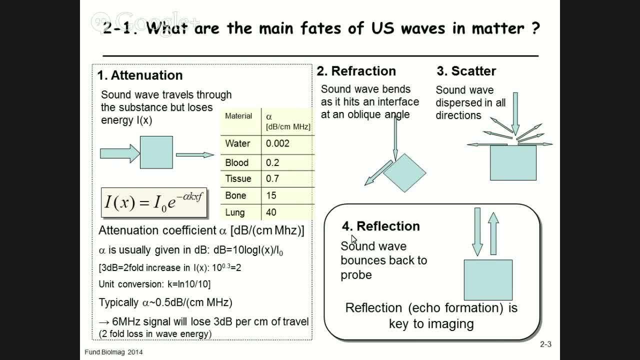 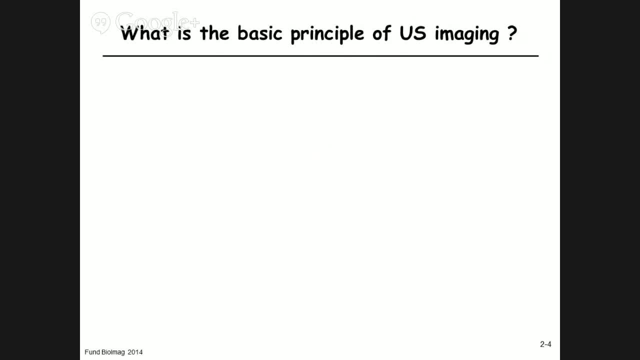 But for the course we're going to deal with attenuation and reflection. The other two we're not going to talk more about. So then, what is the basic principle of ultrasound imaging? So the basic principle is: you emit the sound pulse. 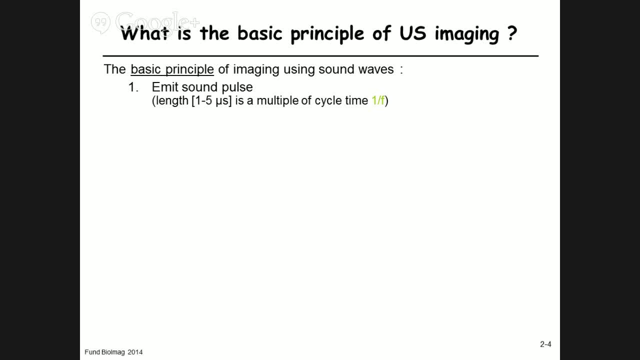 The length has to be, which is typically 1 to 5 microseconds. The length has to be a multiple of the cycle time, That's 1 over the frequency of the ultrasound that one produces. Why does it have to be a multiple? 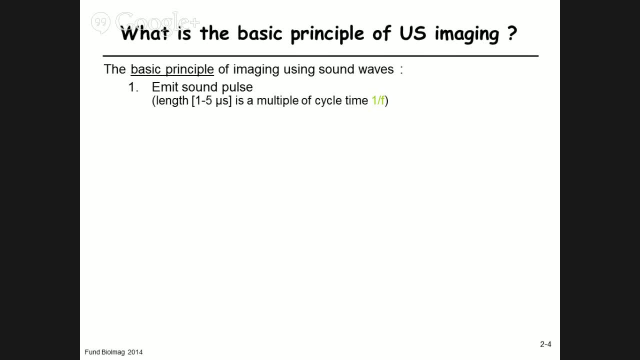 The duration of the ultrasound pulse has to be long enough so that it has a well-defined frequency. If it's too short, then it's the same thing as taking a hammer and knocking it on the table. Then you get the wide spectrum, everything. 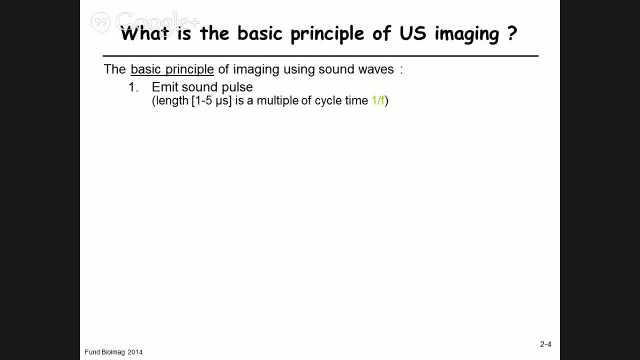 But you want a defined frequency. therefore it has to have a finite length that's sufficiently long that it has a characterized frequency, So some kind of multiple of the frequency. What the multiple is is not so important for us, just to understand the principle. 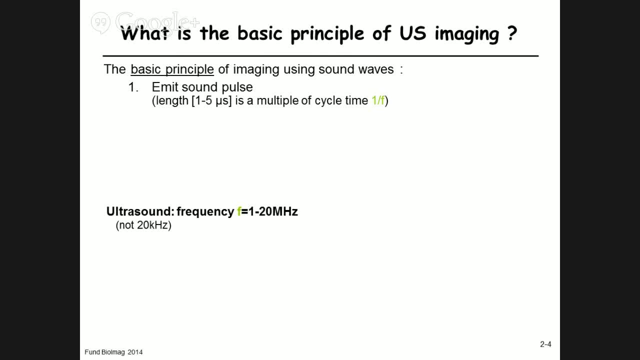 Now, ultrasound frequency for ultrasound imaging is between 1 and 20 megahertz, typically Not 20 kilohertz or 30 kilohertz. We're talking megahertz here. Still, it's ultrasound. Then the next thing that one does after one has emitted the sound pulse: 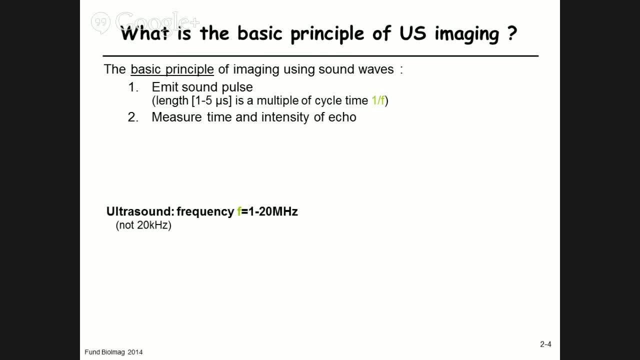 one measures the time and intensity of echo. Many of you have done that before. Certainly those who hike in the mountains essentially Ever heard of lightning. You see the lightning pulse and then you count to know how far away you are from the lightning. 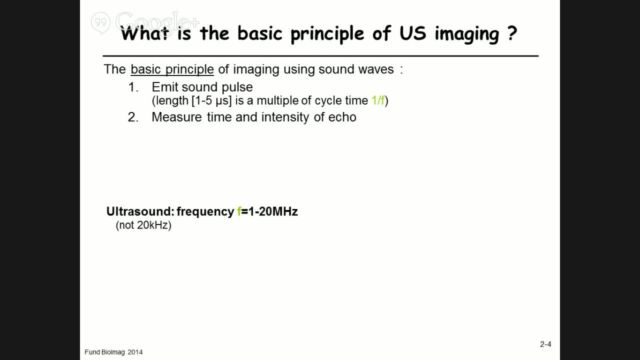 They're using the same thing to calculate the distance of where the lightning was. You have the echo. In this case, it's not an echo, It's just the emitted sound. That's the principle that you're using when you hike. You have a known sound propagation velocity: c. 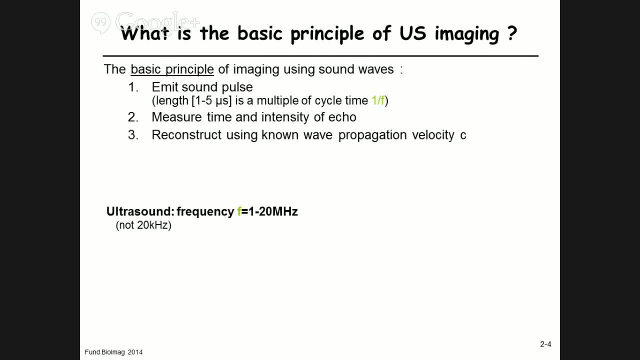 and you can reconstruct then the location of where the echo was produced. Those are, in essence, the three basic principles that underlie ultrasound imaging. I'm going to illustrate this here. Here I've got an object with two different mechanical properties. 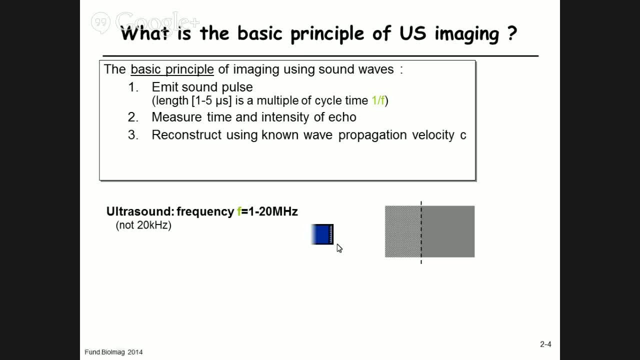 Here's the boundary. It's very abstract. I'm going to attach a transducer to it. The transducer is going to emit sound waves. It's going to be shown here by this little circle That's going to bounce off at this boundary here. 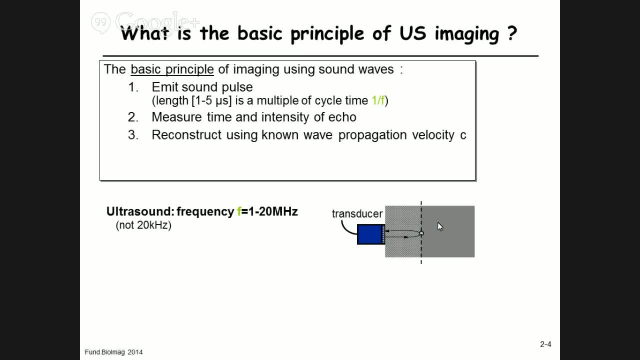 between this tissue and this tissue. The boundary is created just by different mechanical properties. What you do in the mountains: when you holler at a mountain, you've got the boundary between air and rock. Here we're going to have a boundary. 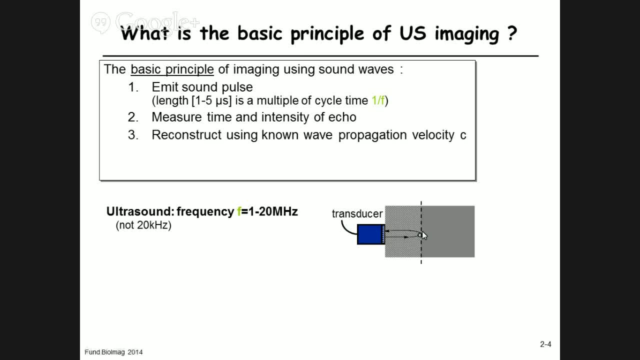 between two different tissue types. The sound wave is emitted and comes back, and from the time and intensity of the echo one can calculate the distance of the boundary from the probe. This distance can be calculated. The distance is very simple, It's speed times the time. 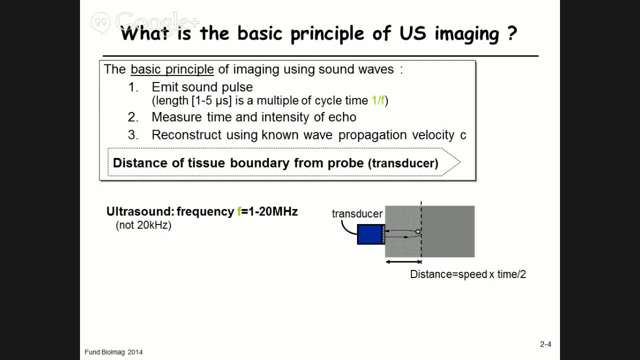 divided by two. The time is the time from the time that the pulse was emitted- That's item number one, the sound pulse- until the echo is received. That's the time. The speed is the propagation, the sound propagation velocity, And we have the factor of two. 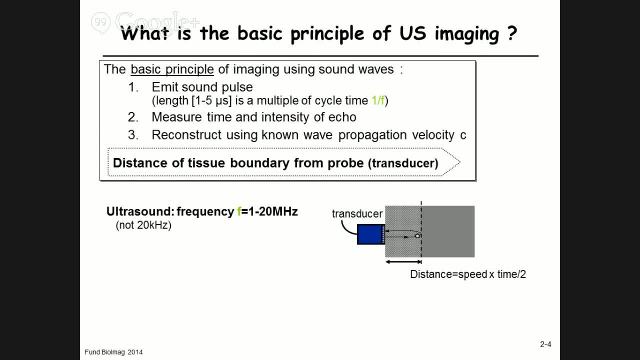 because the sound wave has to go into the tissue and come back, so it travels twice the distance. Okay, so, if you will, the total distance traveled is two times, but what we're interested in is this distance here. So it goes in and back. 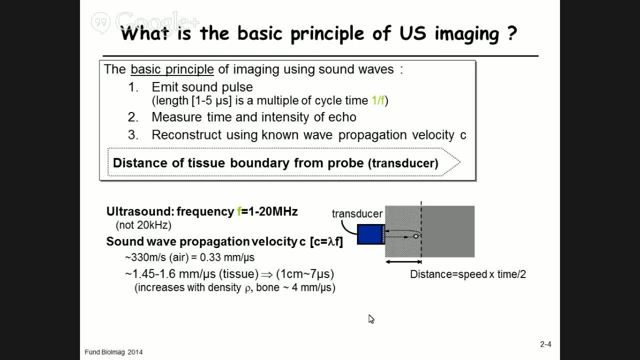 That's why we have the factor two. Now let's get some ideas on the sound propagation velocity In air. it's 330 meters per second, So the lightning three seconds later it's a kilometer away. Convert that to units. 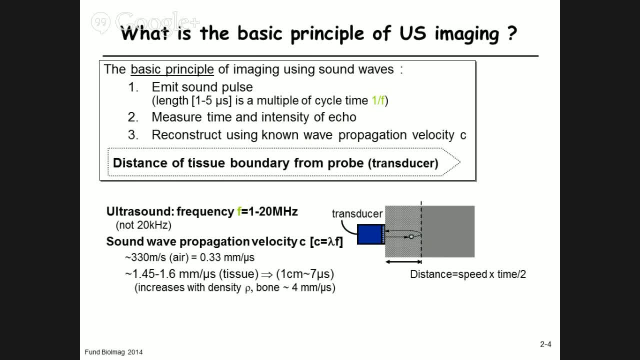 that makes 0.33 millimeters per microsecond. In tissue one has typically around 1.5 millimeters per microsecond, So it's about five times as fast. That means the sound travels one centimeter in seven microseconds. This typically increases with density. 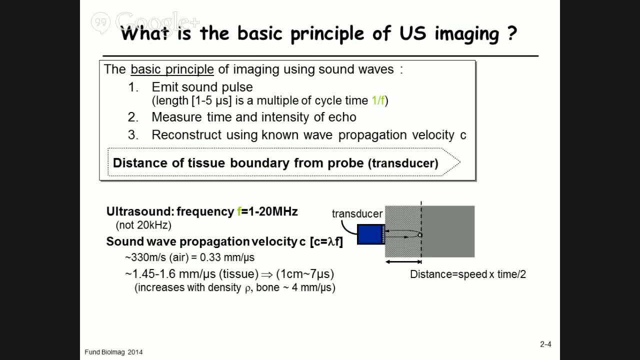 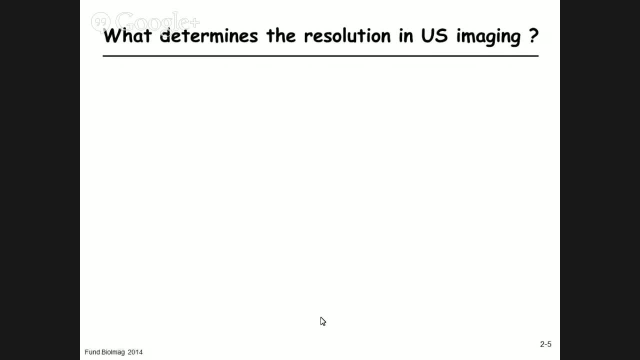 of the tissue row. So in the bone, for example, the sound propagation velocity is four millimeters per microsecond. Okay, so that's the principle. What measures the echo When it arrives, and from that one knows where is that tissue boundary. 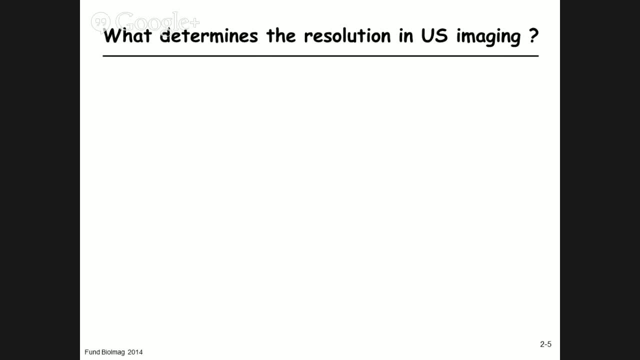 Now, obviously we're not going to have a nice situation, like I just had on the screen, With one tissue boundary. we're going to have many tissue boundaries in the tissue, And so the question is: what determines the resolution in ultrasound imaging? 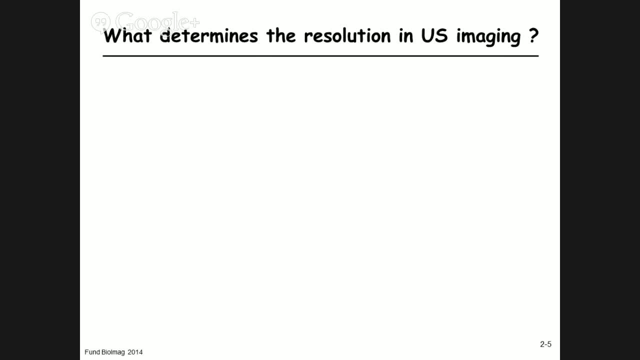 That means what spatial separation of two tissue boundaries can I still separate out with the scanner? And essentially it's the wavelength that determines the minimal resolution, the wavelength of the ultrasound. So I'll illustrate this how the resolution is determined Here. I got the scan head here on the top. 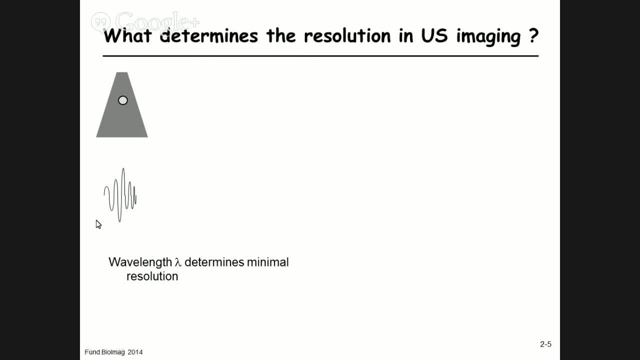 Here it's got one object and it'll produce an echo at this time, the horizontal axis being time, and this is the echo that the scan head has detected. The pulse duration is some kind of multiple of one over f. That is just. 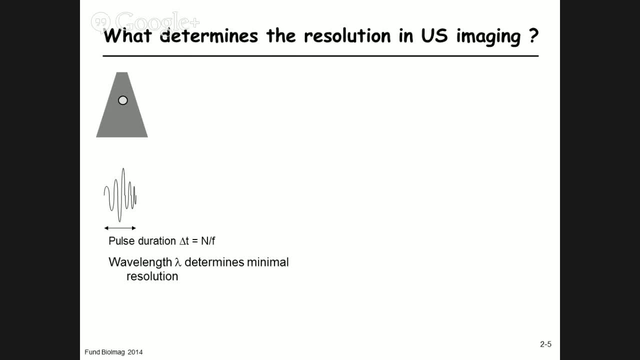 as I said before, to give this ultrasound pulse that's emitted, to give it a well-defined frequency. So this should be n over f should be at least the wavelength or multiples of the wavelength, to have a defined frequency Here it's not so critical. 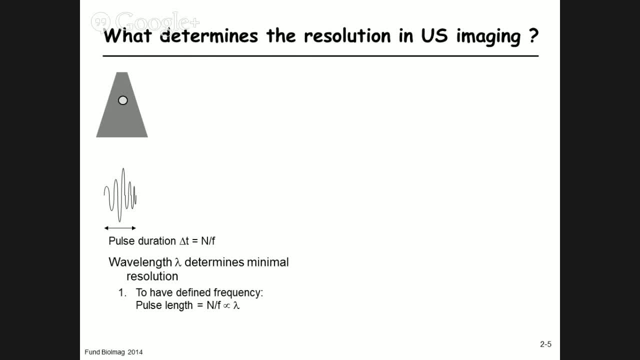 what value is? You're going to have an exercise addressing this, This question, a bit more in detail, but again, the numerical value is the principle that's here important, not the numerical value. So now I have a second object here in the tissue. 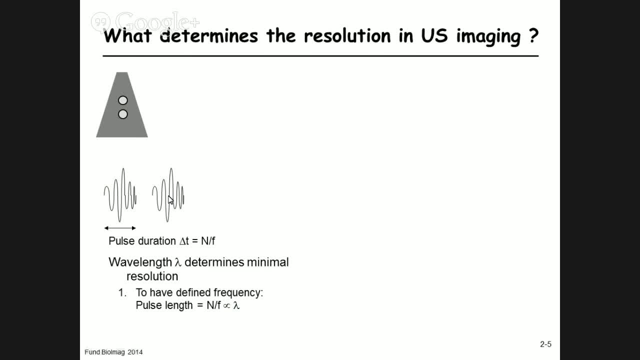 It's further apart and this will now generate, because it's further away, an echo later in time. And if the two objects are well separated, that there's a good gap between them, then we have two separate echoes that come back. 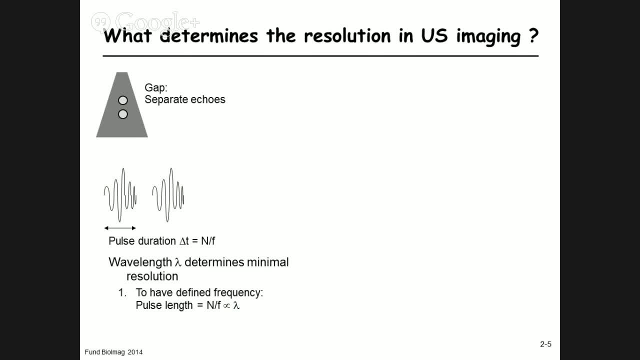 The scanner can digitize them, recognize them with the software and say: I've got two distinct echoes, The two objects are at two different places and everything is nice and dandy and we're good. Now we need a minimum echo separation here. 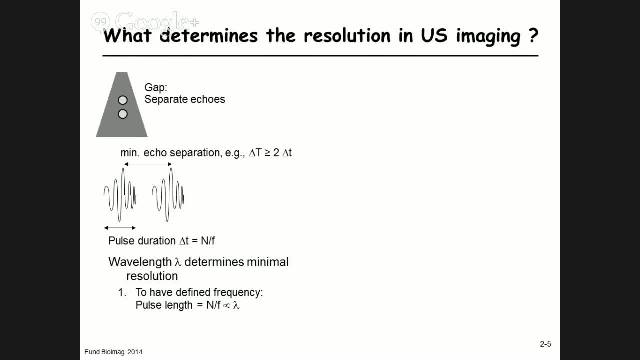 Something like a delta t that should be bigger than two times small delta t, where delta small t is the length of each pulse. Okay, this could be two times. this could be three times. Again, the numerical value is not critical, It's the principle here that's important. 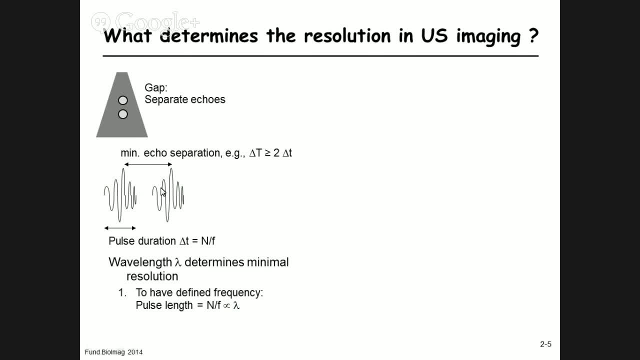 Why is that? Because we need to give the algorithm a chance to say: well, I've got two different echoes, I've got two different maxima here, I've got two different events, And that the computer can separate them. So that leads us to a separation. 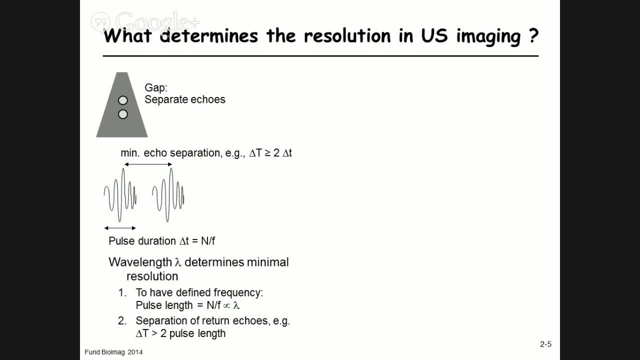 of the return echoes, and probably the minimum is around two times the pulse length. Okay, so let's now consider again an object. Same situation. Scan head is up here. Here's my object: Produces an echo in time here. 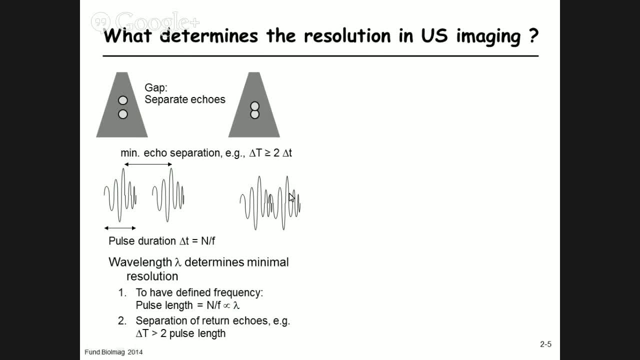 And I've got a second object which is closer, And this will produce a second echo that's closer to the first one, because they are closer to each other. So the second echo will arrive shortly after the first echo from the first object. 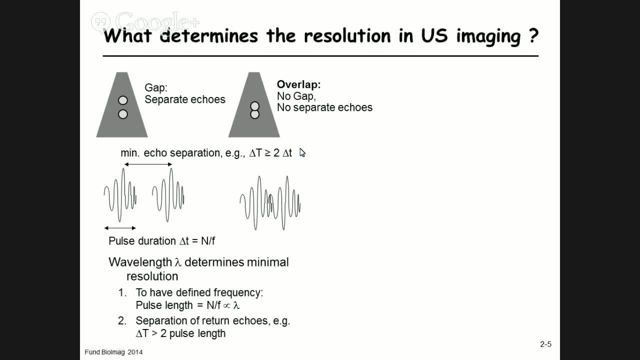 Okay, so if we have overlap, we have no gap, We have no separate echoes. So what happens If we start overlapping the objects? if they're closer, then now you've got a signal that looks like this: The echo from the second object. 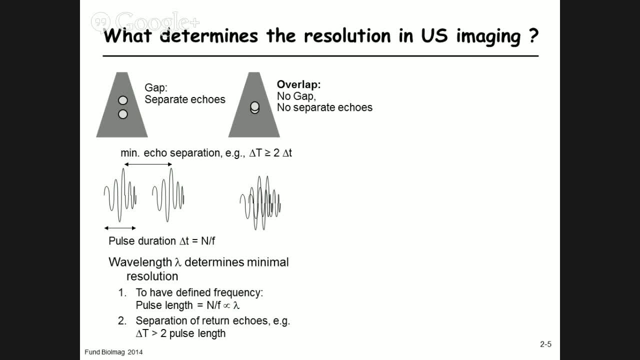 is slightly shifted, but no longer enough that the software can distinguish the two echoes. It will treat this as one echo, And so at that point the scanner is no longer able to separate out the two objects, and the resolution is lost. So basically, 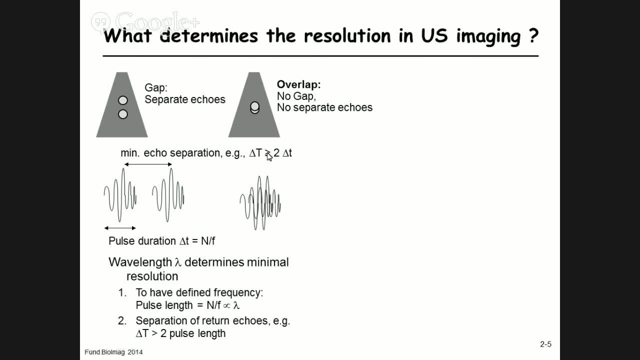 one needs to have a certain separation and that means a certain minimum time between the echoes. This minimum time, through the equation of distance, equals speed, velocity times. time divided by two gives us a minimum separation. spatial separation, that's possible. Okay, so if we look at the echo, 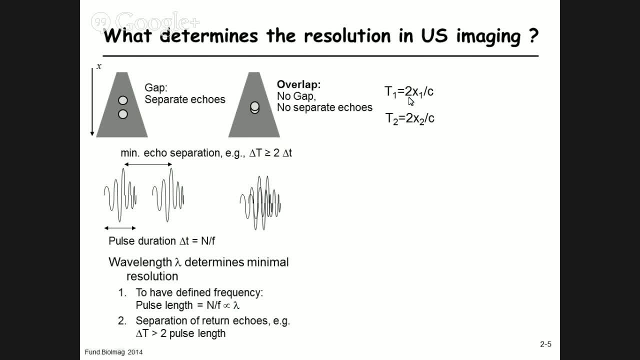 the echo one arrives at 2x1 over c. c is the wave propagation velocity t2 for the second object at 2x2 over c. So the delta t is now two times delta x over c. so the delta t here defines: 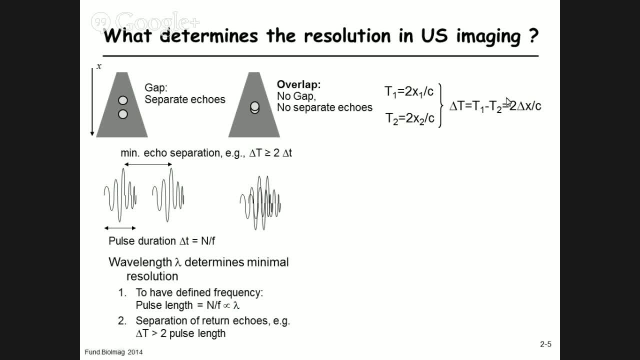 the delta x. the minimum delta t that one can resolve defines the minimum delta x of two objects that one can separate out. Okay, so what is the conclusion here? One conclusion is: resolution increases with frequency. Why is that? Because as the frequency increases, 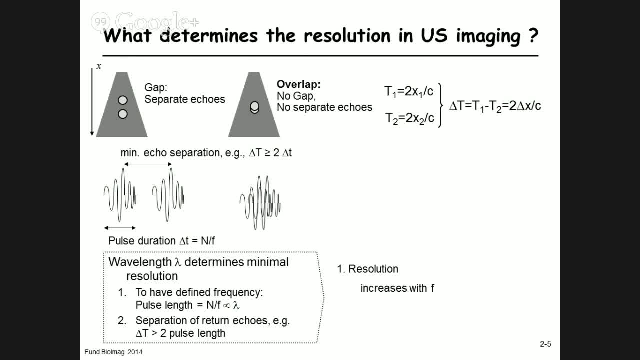 one can reduce the duration of the pulse. If one can reduce the duration of the pulse, one can reduce the delta big T of the separation of the two echoes. If I have two very sharp pulses sent out, think of it as two delta distributions. 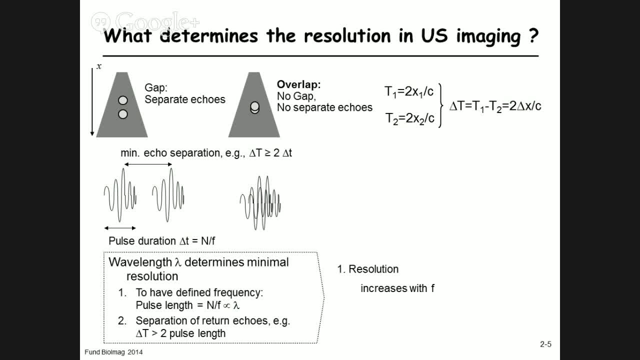 Okay, if that you could do- which we can't, but let's assume you could- then you could have an infinitely high spatial resolution, And that's just a matter of thinking. if the frequency is lower, then the pulse duration has to get longer. 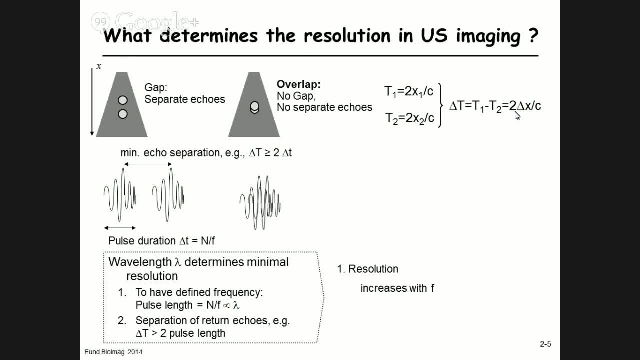 and then the minimum separation of the two echoes. the delta t here has to increase. So resolution increases with increasing frequency. However, penetration- that's what we called attenuation before attenuation- decreases with frequency. So ideally one would like to have a high resolution image. 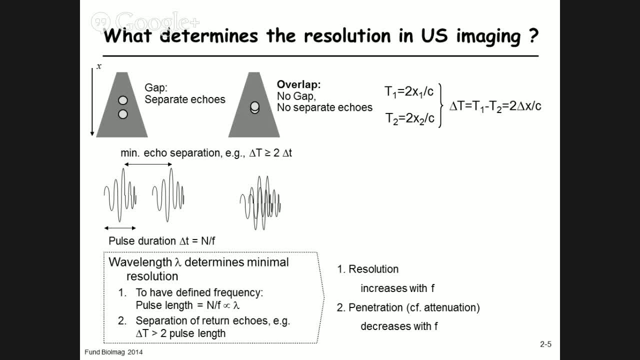 with ultrasound. so one would increase on the knob, increase the frequency, go higher, but as one does that, the attenuation increases as well and the signal gets weaker And at some point all that one records is just noise. So we're back to the old principle. 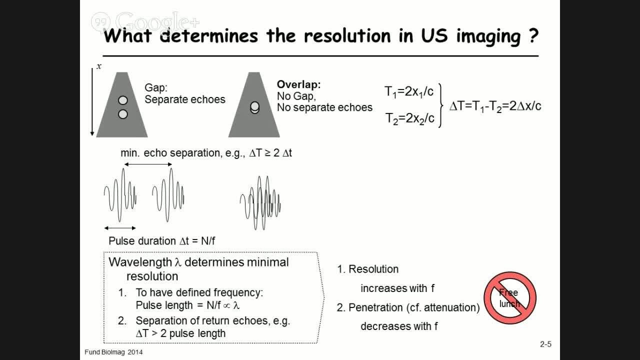 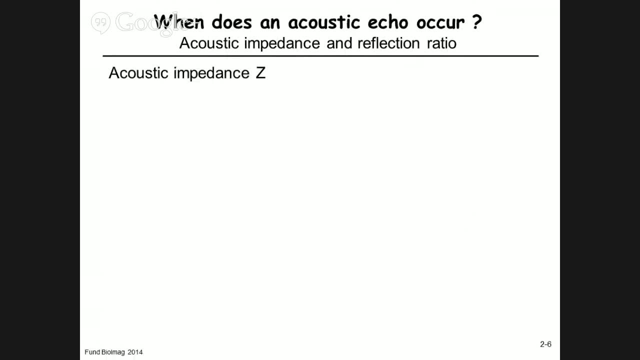 that in biomedical imaging, as in life, there is no free lunch. There's always a trade-off between one or the other, And here that's very obvious, with the frequency, the effect of frequency. Okay, so when does an acoustic echo occur? 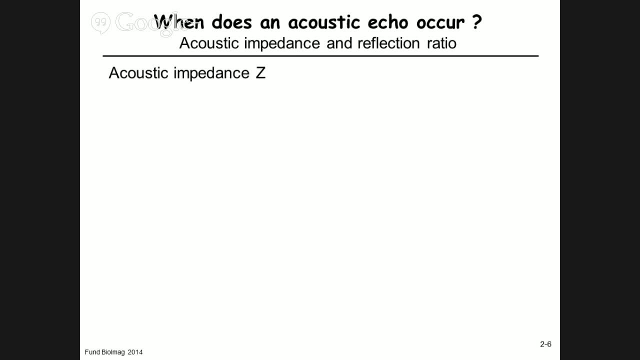 We're not going to deal with too much with the biophysical details that underlie this. I'm going to be very empirical in this and introduce the term of acoustic impedance, which is given by: z equals the density times the velocity, speed, velocity. 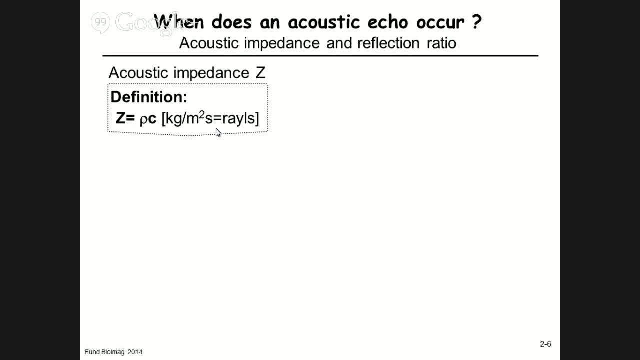 These are the units and instead of writing all this stuff here, one calls them rails. Don't know why they call them rails. Probably some Mr Rail invented them. This is to give you some idea of what is the variation in acoustic impedance. 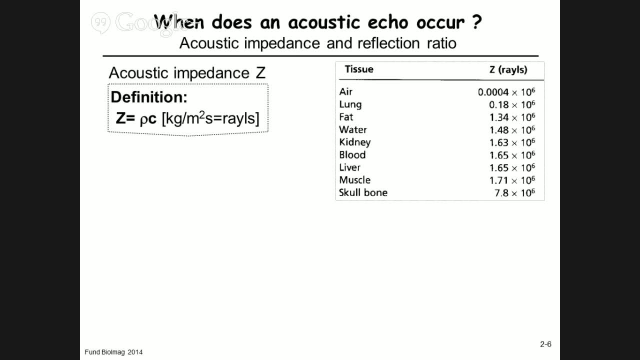 between different tissues. You have air which is very low. You have lung a bit higher. Lung is not just pure air. Then fat, water, kidney, blood, liver, muscle- They're all about the same. And then you've got skull bone. 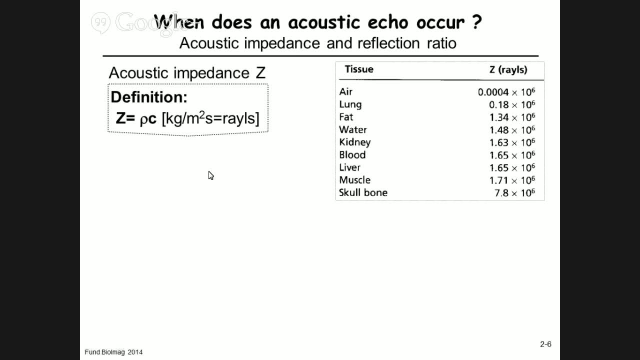 which is substantially higher than the others, about a factor of five. So, but from the acoustic impedance which is a property of the tissue- its stiffness if you will- one can deduce the amount of reflected wave energy, And this is given by the initial intensity. 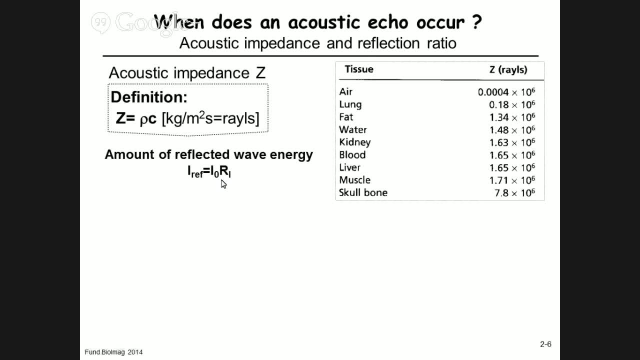 times the reflection coefficients, coefficient r here. That gives you the reflected intensity. So what defines the occurrence of an acoustic echo is that one needs to have two different tissues with different mechanical properties, ie two different acoustic impedances, and this will give us the echo formation. 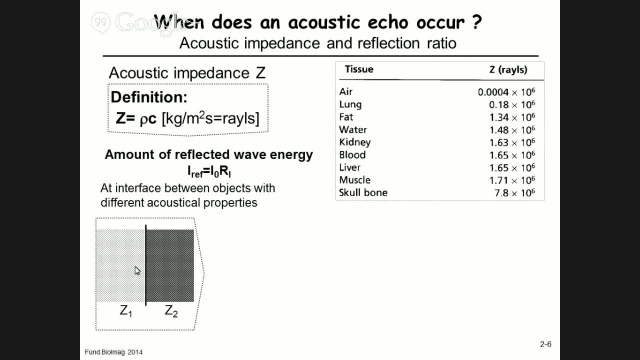 So here I've got a simplified object with an acoustic impedance, z1, and another tissue with z2.. And the reflection coefficient is given by this equation. here It's the difference of the acoustic impedance divided by the sum of the acoustic impedance squared. That's the reflection coefficient. 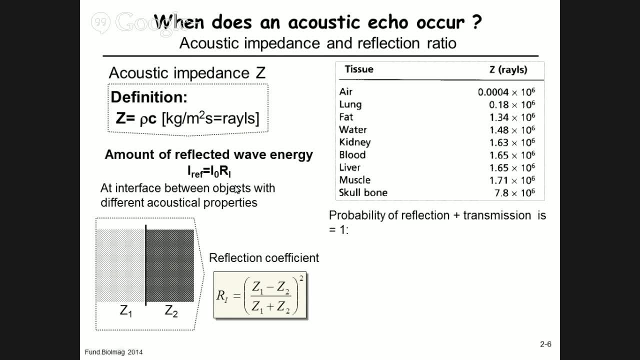 that tells us how much, what percentage of the acoustic wave is reflected. Now, neglecting all the other facts, the probability of reflection and transmission is one, So we can calculate the transmission coefficient. this is just one minus r, the reflection coefficient. 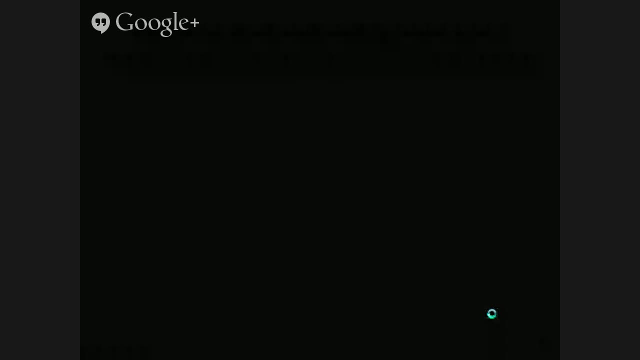 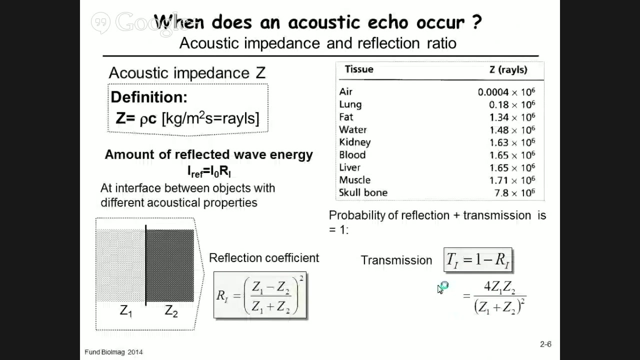 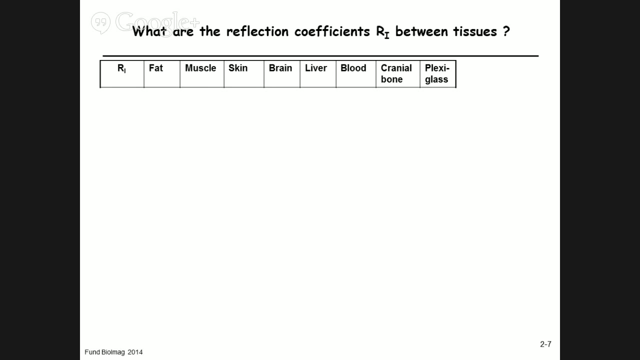 and if one does that and does the math, one obtains this expression here. So that's the transmission coefficient here. Okay, so now what are the different reflection coefficients between different tissues? Giving you a list here of different tissues, because we have had on the previous slide. 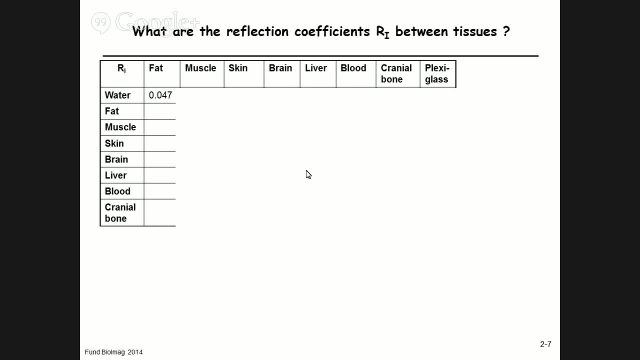 some ideas of the acoustic impedance And we're going to just look at. between fat and water the reflection coefficient is 0.47.. This means about 5% of the energy is bouncing back. Then we've got muscle and water. 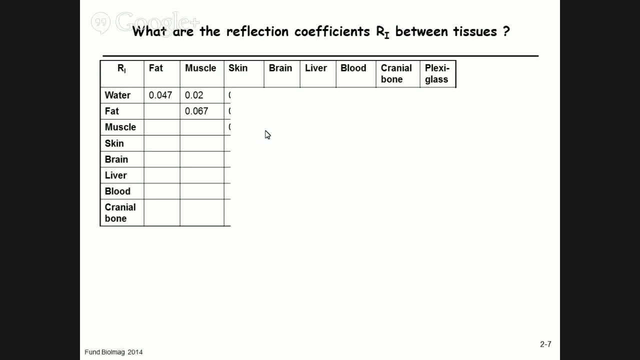 muscle and fat between 2 and 7%. Skin fat versus water fat and muscle it's between 1 and 8%. Here is brain, liver and blood. You get the idea. They're awfully low. It's not a lot of echo that comes back. 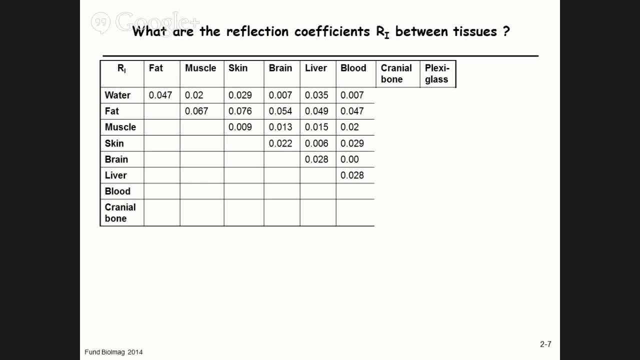 Imagine you're in the mountains, you do your nice song, like they do the shepherds in the mountains, and there is only 2% of the echo that comes back. That's a lot of hollering that you have to do to get something back. 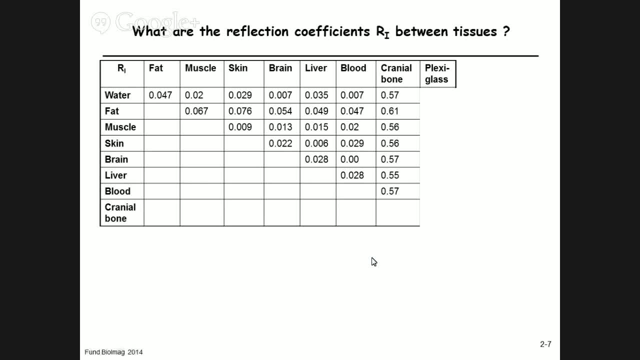 Okay, but that's the fact. Then we go cranial bone and now we're in 50-60% range of reflected energy and plexiglass is in the order of 33%. Okay, so what does that mean? 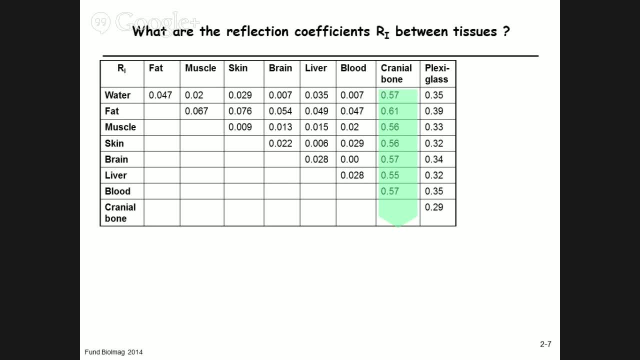 Cranial bone is so high. What's the consequence of having such a high reflection of the solid versus soft tissue? It means when you have solid material, you have a lot of reflection of the sound waves, For example, bone-tissue interface. 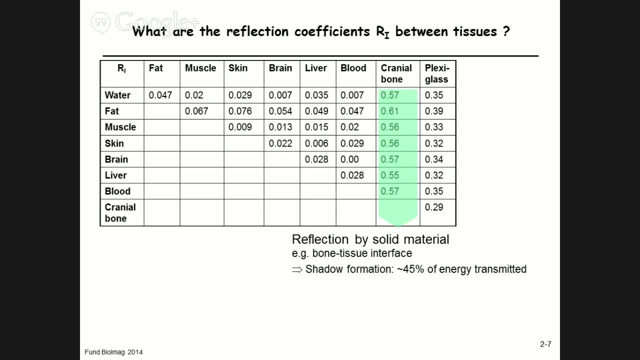 And that produces an artifact in the images which is called shadow formation. Okay, let's say you want to look at a lesion behind the bone. You send out the ultrasound, but 60% of the signal is reflected, so only 40% goes through. 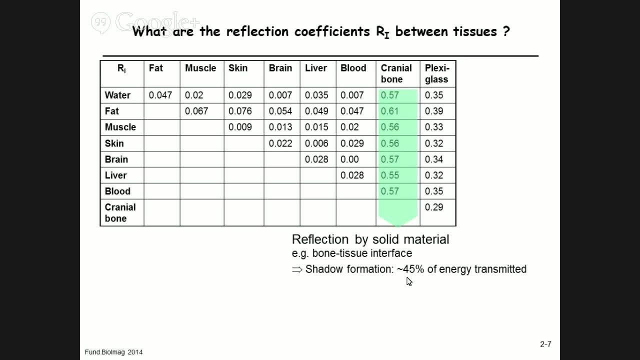 So there's a 60% reduction in intensity. In this case it means only 45% of the energy passes the cranial bone. So I'm going to illustrate this principle, but first, before I do so, I'll give you an example here. 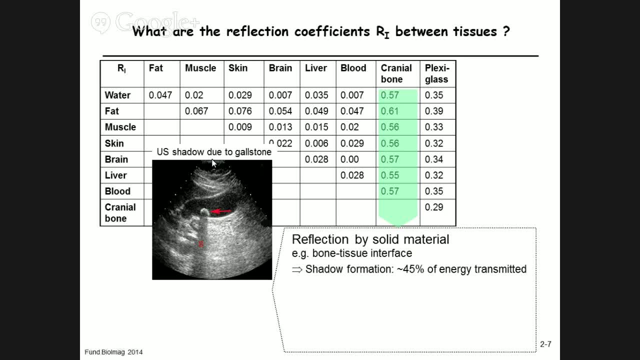 This is the gallbladder. This is a gallstone. The ultrasound is up here. What happens is the gallstone is solid material, so there's a lot of the wave energy is reflected. Because the amplitude is high, it shows up as a very high signal. 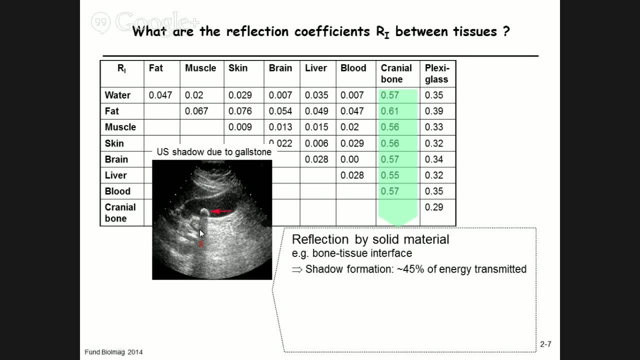 But this energy is missing down here, and so you've got the shadow formation behind the gallstone, where you lost intensity and therefore ability to detect lesions. So how does this happen? So let's assume I've got bone here. I'll just take the example of bone. 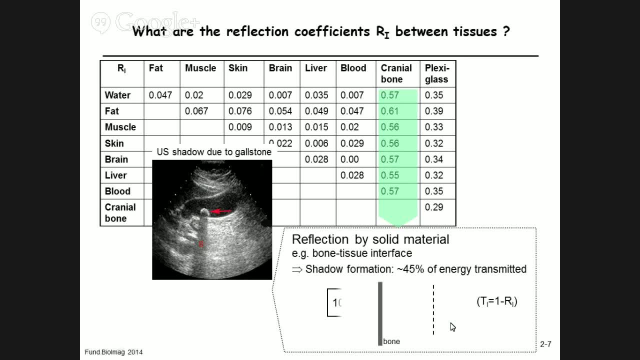 I've got some tissue boundary that one would like to image here And we have an incoming wave at 100%. Only 45% goes on. Let's assume it's perfectly reflected at this boundary. That's the perfect case, And 45% comes back. 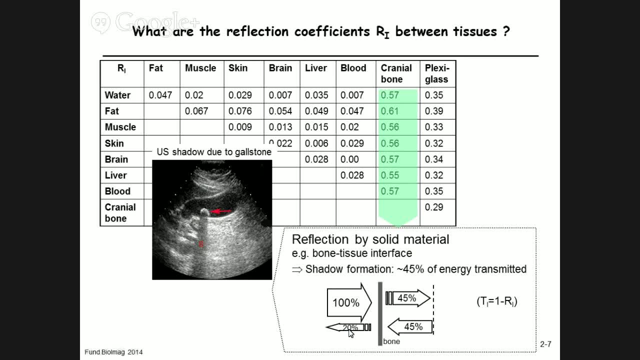 but again, only 45% passes. It passes through the bone, so in the end you have only 20% of the signal And that's why you've got this shadow here in this case. Here's another example from the video I showed you last week. 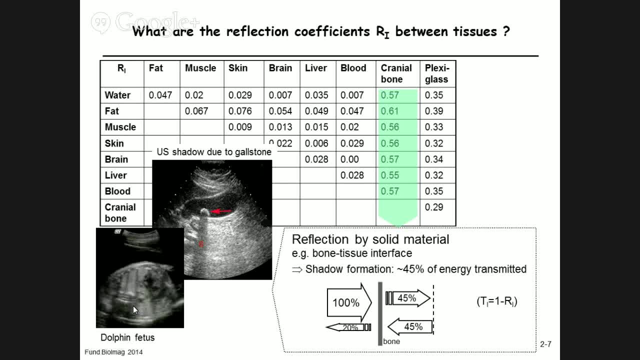 That's from the dolphin fetus And you can see these streaking artifacts here. The scan head is up here, This is the uterus and here is the fetus. These streaking artifacts correspond to the bones of the rib cage, Each one of the bones. 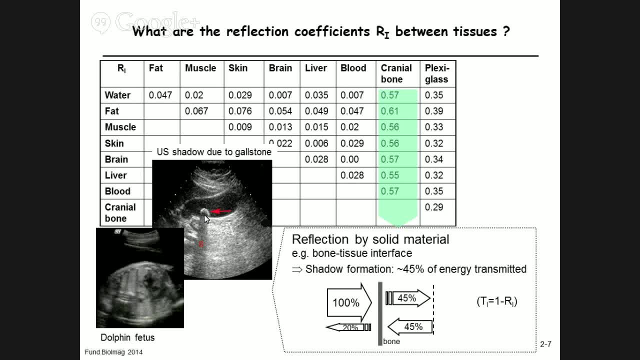 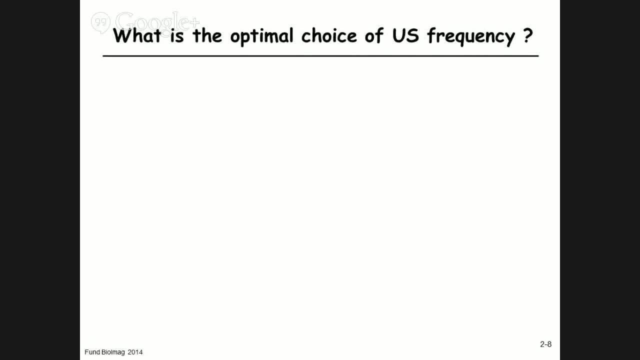 reflects the energy, and so it produces the shadow formation, just like the gallstone here. Okay, So we have seen that for ultrasound imaging, one is caught between two desires: the desire to have a high frequency and the desire to have low attenuation. 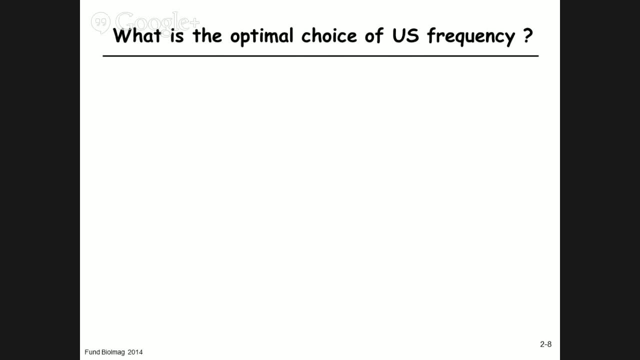 That is a low frequency. So there must be, for an application, an optimal frequency, And this is what we're going to address here. So we have, when we have increased resolution, we have decreased signal-to-noise ratio because we have attenuation. 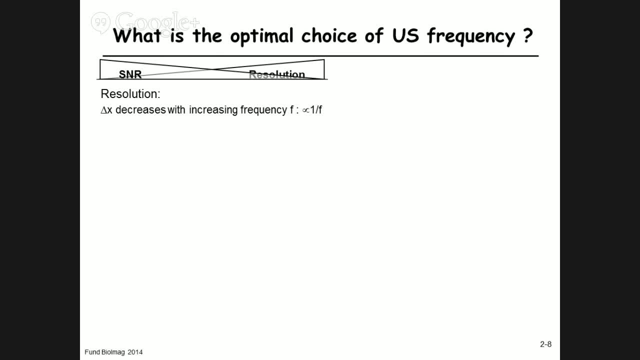 So delta x. we have seen decreases with increasing frequency. So the resolution goes inversely proportional to the frequency. I mean the delta x. So the resolution we can say increases with frequency Signal-to-noise ratio. that is the attenuation. 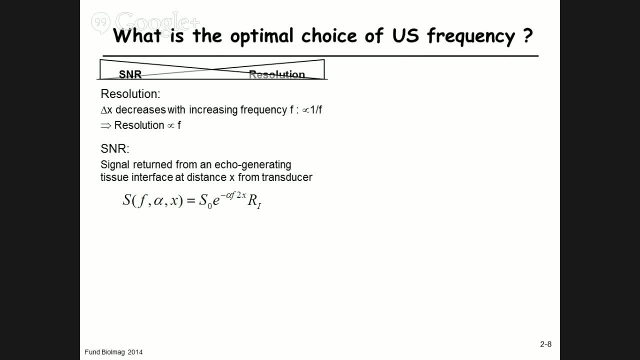 is given by the attenuation equation that we used before, that I introduced earlier. And then we have, of course, the reflection coefficient here. Okay, So that is the signal that's returned from an echo-generating interface. Just note: here we've got 2x. 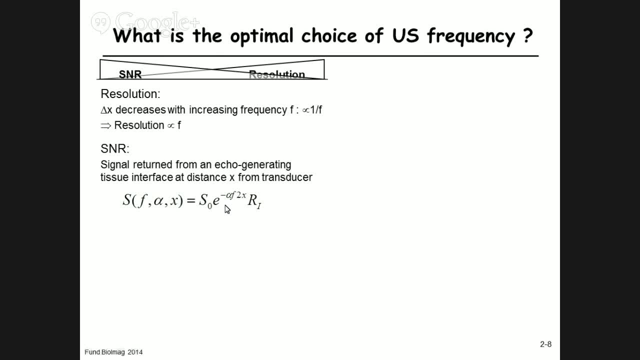 and the factor k I forgot to put in here. I'll have to change that. That's the conversion factor between decibels and the exponent. So Okay, So the reflection coefficient as a function of frequency is constant. F is the ultrasound frequency. 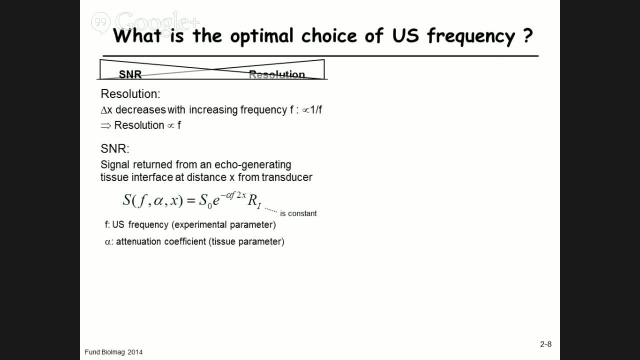 And I will come back to what I introduced last week- This kind of behavior analysis on when is the optimal choice of our experimental parameter. And F, the ultrasound frequency, is the experimental parameter, That's the parameter that one as an experimenter can choose. 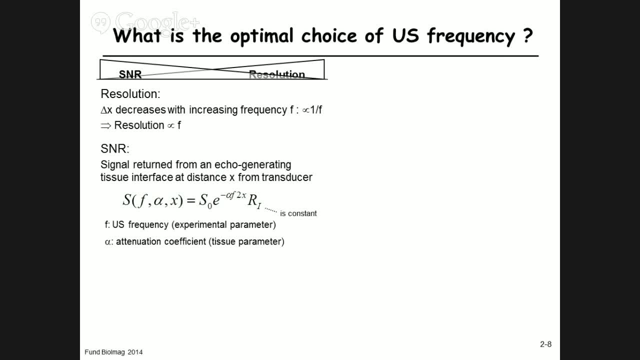 1 to 20 megahertz, or whatever. Alpha is the attenuation coefficient, That's the tissue property parameter, That's the one we cannot change, That's the one that's given by the subject under investigation. So now the question is: 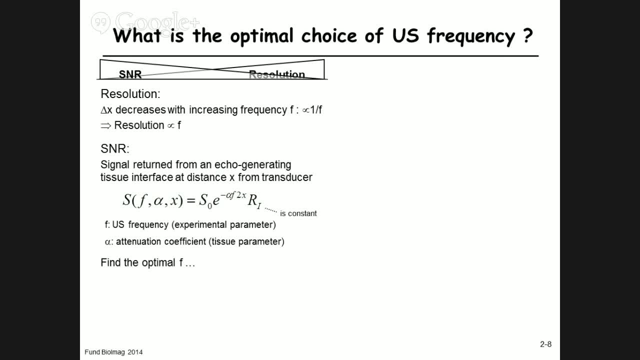 one would like to increase the frequency, but one would like to decrease this term here, And so there must be a choice, an optimal between the two, And the idea now here is we're going to take the signal that we want to maximize. 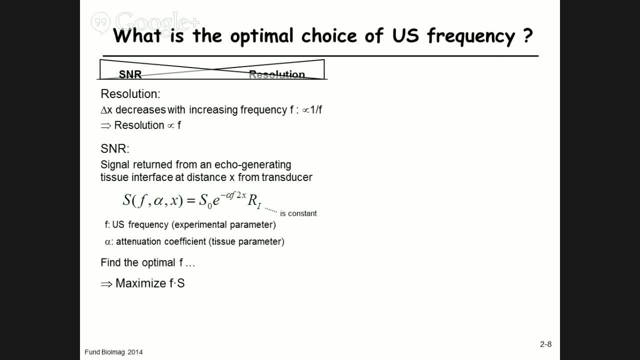 and the frequency that we want to maximize. So let's maximize the product of the two. Okay, now you could say: why are you maximizing F times S and not F squared times S or so? Because I can. It's arbitrary, But you can actually go through the calculation. 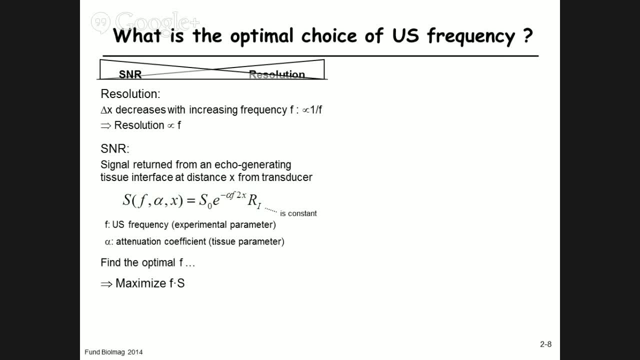 and ask the question: what if I give more weight to the resolution and I maximize F squared times S, And you'll find very similar behavior. Okay, so now we want to see where is the maximum where the derivative with respect to the frequency is zero. 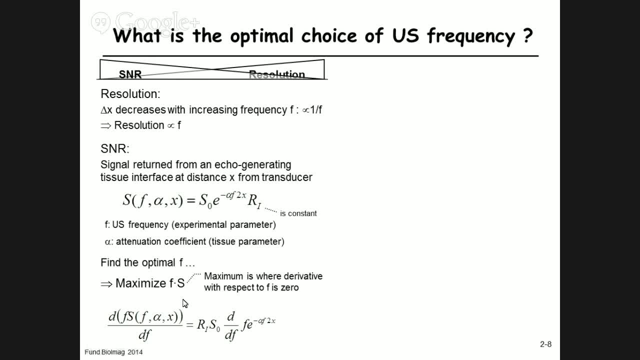 That's the maximum, the best frequency we choose. So we multiply F times S- S is a function of these parameters- And then take the derivative with respect to the frequency. Here is the constant sort taken out. We have the derivative of this guy here. 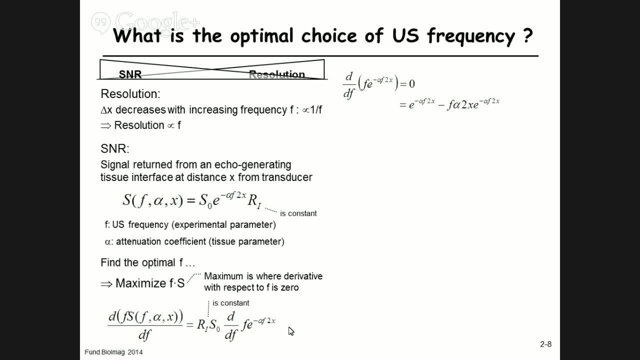 And so we're just going to have to look at the derivative of this. We'll just spare ourselves the details here, But here is what we get: The exponent stays in both expressions. We've got something in brackets that we can set to zero, which is nice. 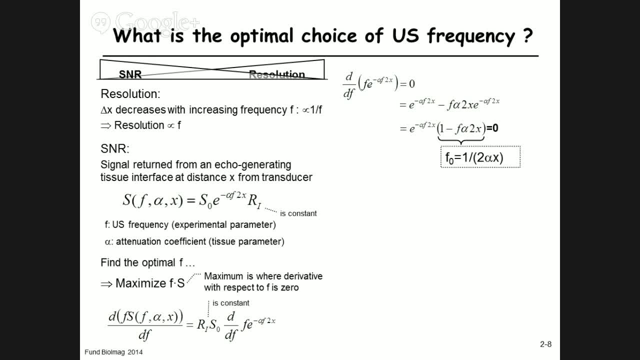 So we're finding the optimal frequency is given by one over two times the attenuation coefficient and the distance of the object with respect to the transducer. The two is, of course, because it travels back and forth. Okay, so the frequency, the less attenuation we have. 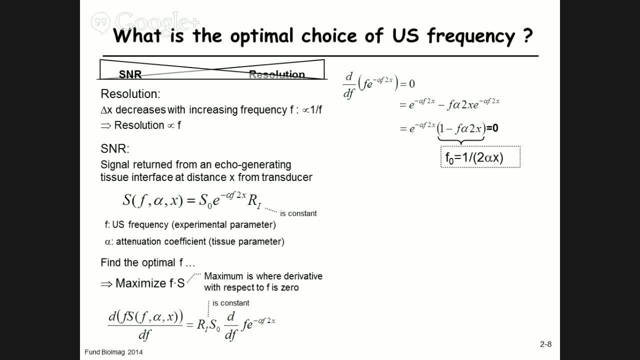 the higher the frequency can be chosen. That's the right behavior. The further away the object is, the lower the frequency has to be, because one has to have less attenuation. And the further the object is away, the more attenuation one has. So this result makes intuitive sense. 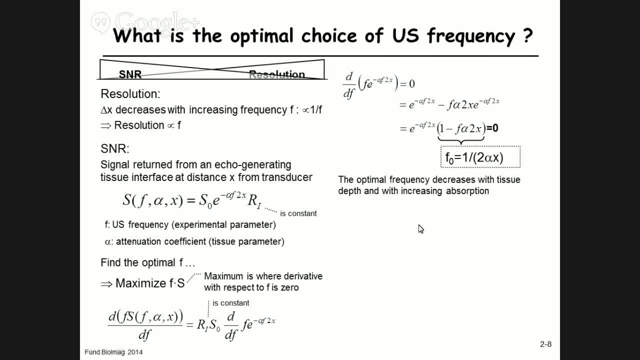 So that's what I just said. The optimal frequency decreases with tissue depth and increases with increasing absorption. So let's look at this function and let's see how critical this choice of F zero is. I'm going to pretend here the experimenter has chosen a certain F zero. 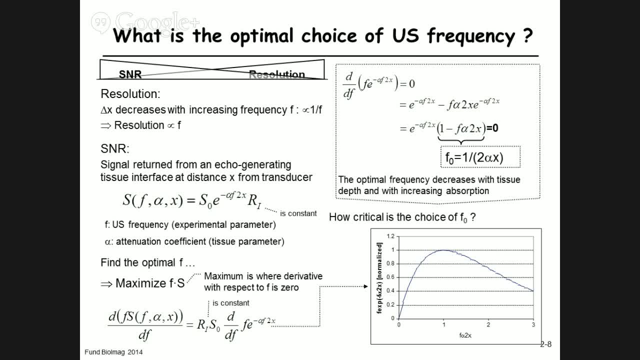 and the question is now: how much an error can one allow oneself in knowing what is the attenuation coefficient and the depth? And so what I've plotted here is this function, here as a function of F, alpha two, x, and this gives us this curve here. 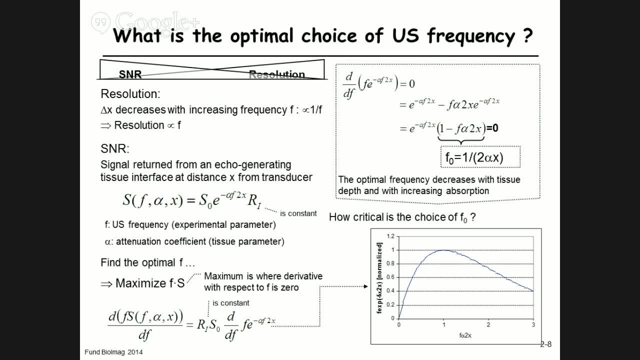 This actually looks very similar to what we've seen last week and you'll notice. actually it's an exponent that's involved. Here's the optimum. This is a normalized to one, So at the optimum I set this equation to one. That's just scaling. 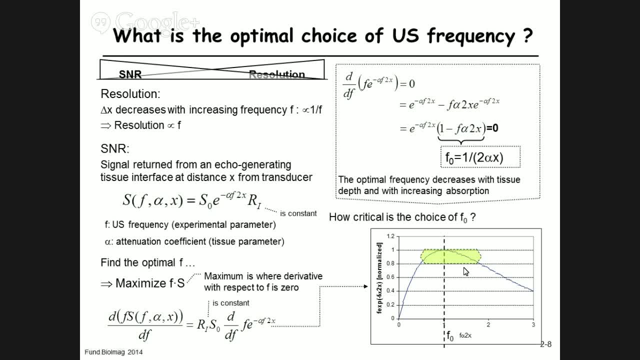 And now you can see here we got a certain variation within 80%. and if one decides, I'm okay if my signal is attenuated by 20%, then if I still receive 80% of the signal, I'm still happy with that. and that gives us now the range of frequencies. 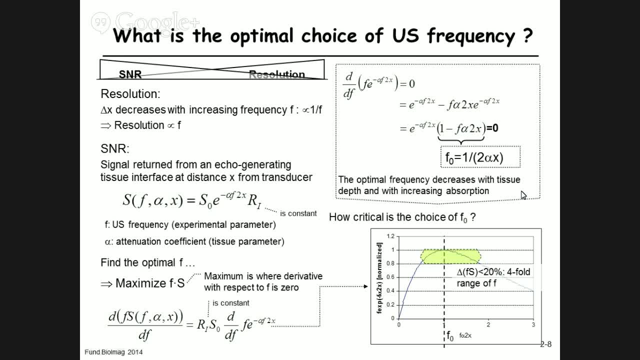 that one can accept. So if the change in F times S is less than 20%, one gets a fourfold range of frequency. So the good news is, if the distance varies by a factor of two, you can still use the same frequency. or if the attenuation coefficient varies. 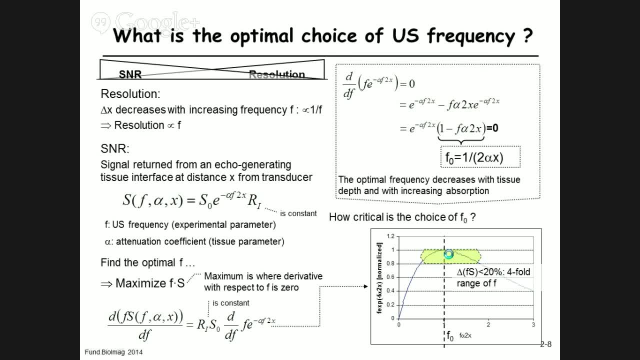 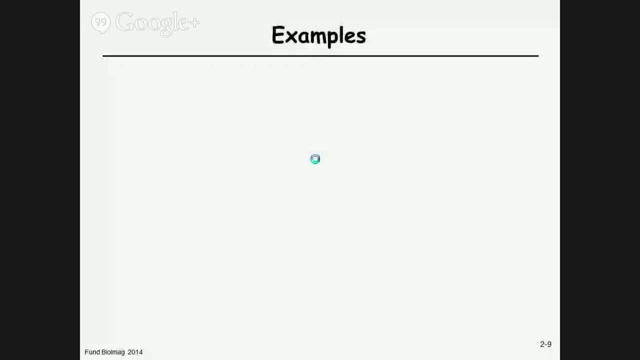 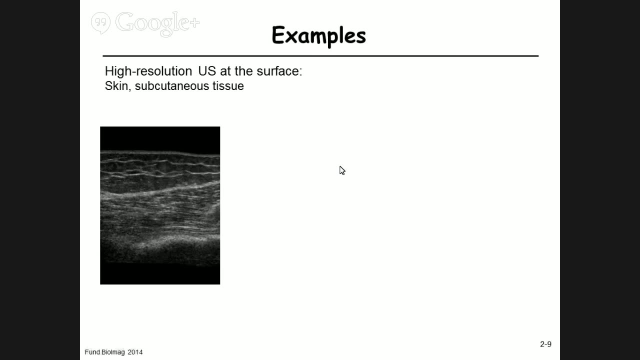 by a factor of two, you can still use the same optimal frequency for a given distance. Okay, So now let's look at some examples that illustrate the principle. So the first one is a skin ultrasound, Very high resolution. This is you know. 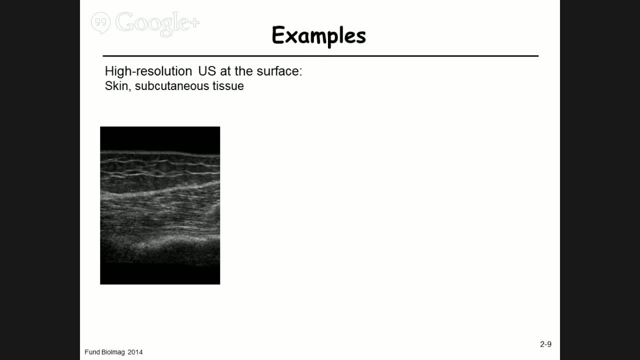 that's the problem with ultrasound: You have to know what you're looking at. It's just kind of circular as far as I'm concerned. What you see here is the epidermis, That's the surface. You have loose connective tissue. 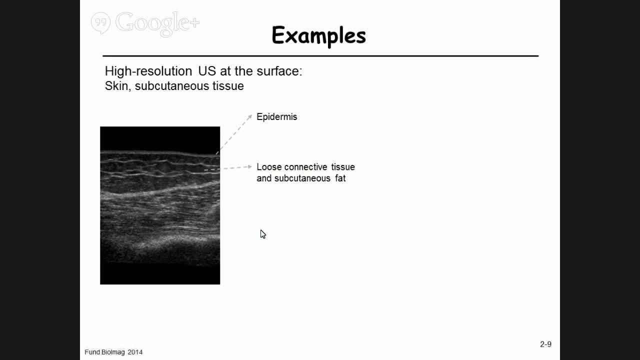 and subcutaneous fat. That's the next layer. Then here that's the muscle-fat interface. This is striated muscle Muscle fibers interface. You can actually see here the individual muscle fibers, It's so high resolution. And then down here one has the bone. 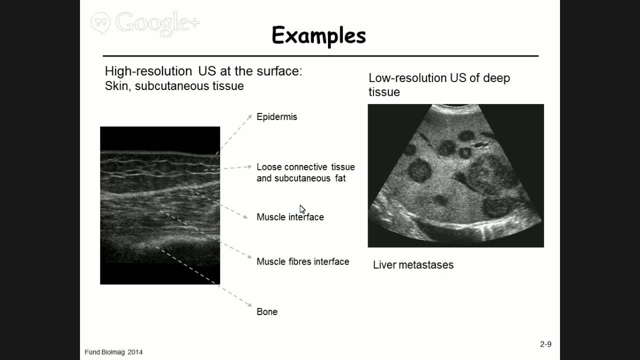 So that's very high resolution if you can see the individual fibers. But if you want to look at liver metastasis, which are many centimeters away in the human liver, the liver has about a weight of one and a half kilos, so you can estimate the size from this. 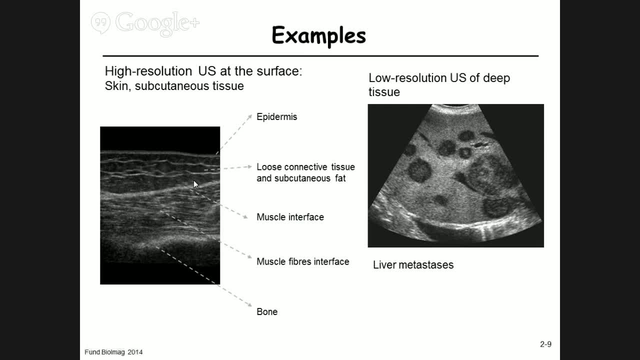 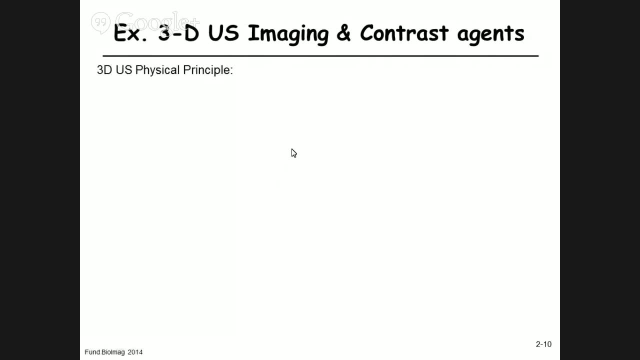 You see the metastasis. There's no chance that you would ever have this kind of resolution For this scan. So here the frequency was low and here the frequency was very high. Okay, Now further examples. 3D ultrasound: I am not going to go into all the math. 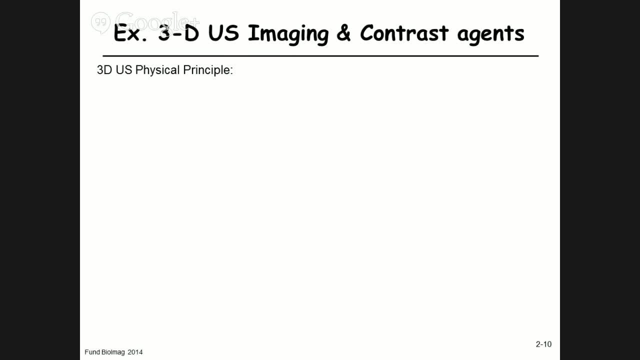 of how an image is reconstructed, just to give you a gist of the principle that's being used. During the scan, the transducer is moved, So you give it a linear shift, swinging or rotation. The received echoes are then stored in memory and based on the movement of the head. 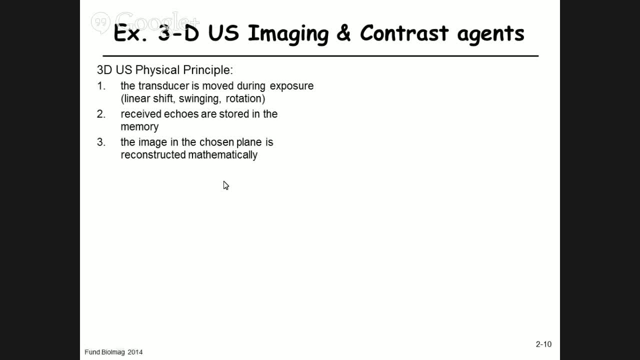 that is being done. the image is reconstructed mathematically, So that's roughly the principle here. This is what a 2D image looks like of a fetus. here You can see the head, the nose, the hand is here And that's the umbilical cord here. 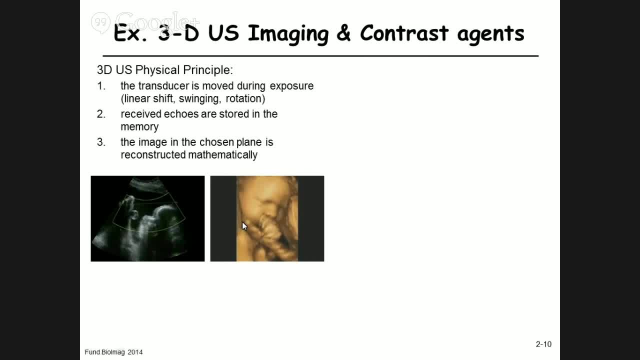 You can see the three vessels that are in there And this is the corresponding three-dimensional reconstruction. Very nice image of this unborn child And that's the umbilical cord here. That's just the cross section. The nice thing about ultrasound is: 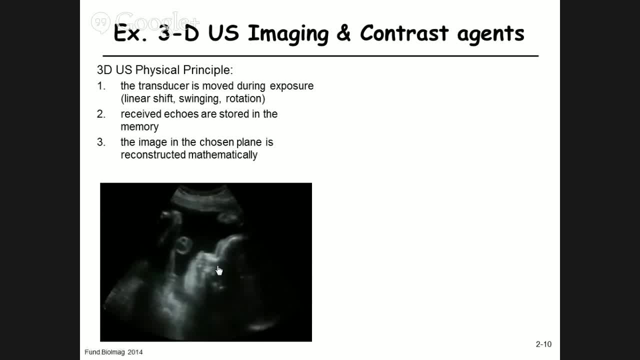 that you can actually watch images in real time. So this is now the baby moving in the womb, The umbilical cord. Now they select the area for the 3D reconstruction here And that is now the three-dimensional reconstruction And the heartbeat that one can see. 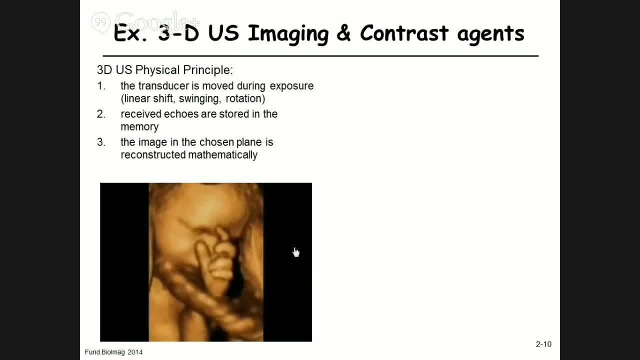 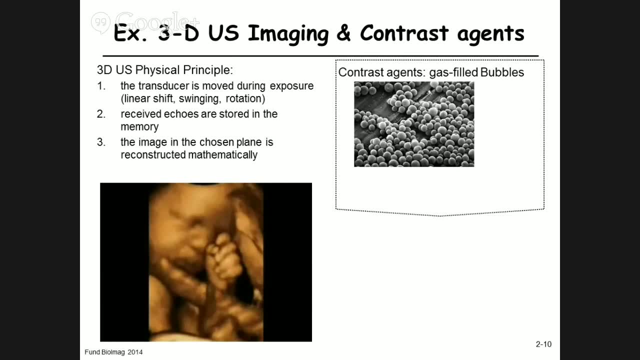 You can see even the toes, the nails on the fingers. Okay, Contrast agents. We're going to talk about contrast agents. What they are done. they're actually being developed in Geneva and Bracco. So they are gas-filled bubbles, Little bubbles. 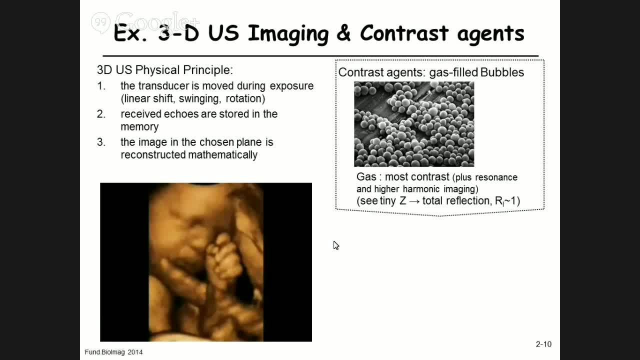 That produce A more contrast. So and then, on top of that, you have resonance. The gas bubbles will go into resonance And this allows for a thing called higher harmonic imaging. And because it's gas, it has a tiny z And therefore you have total reflection. 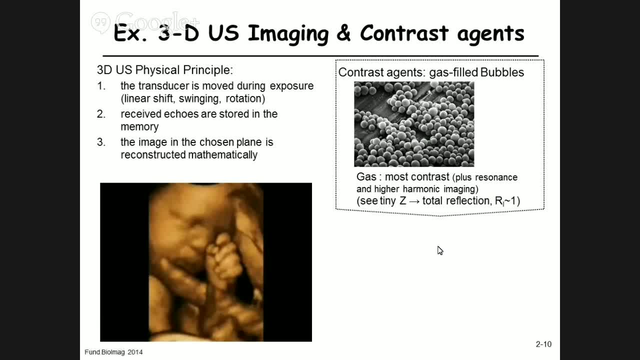 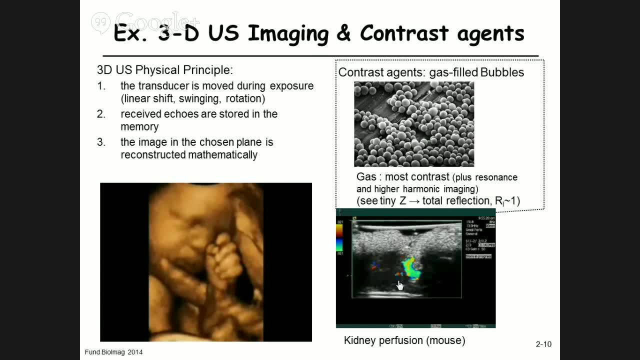 Reflection coefficient of one, So it gives a very strong signal. That's just the principle of what the contrast agent for ultrasound looks like, And this is now an example of a kidney perfusion study in the mouse. So here's going to be the kidney. 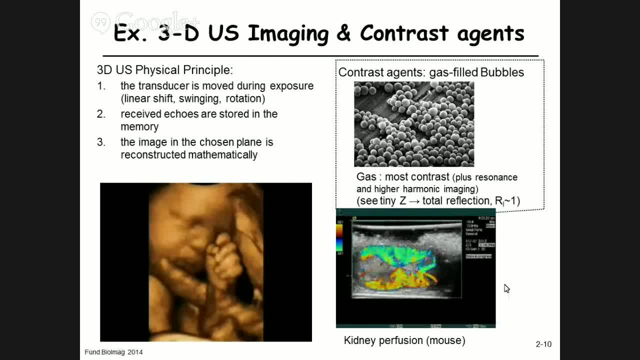 What we're going to see. You're going to see the injection of the contrast agent And the signal that appears is now color-coded And you see very nicely the cortex of the kidney here: How the contrast agent in the blood through the circulation. 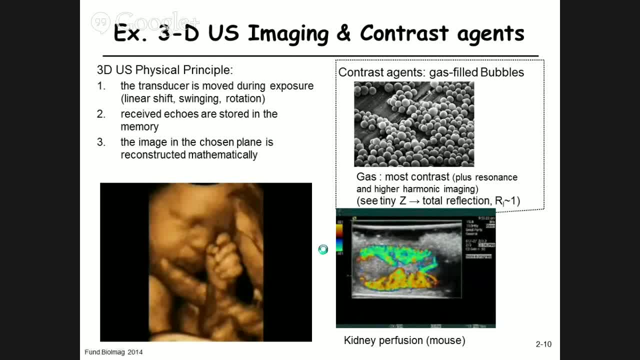 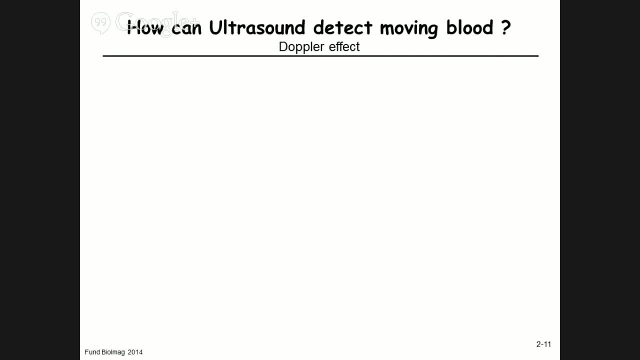 ends up in the cortex of the kidney. Okay, Now the last one is: how can ultrasound detect moving blood? And that is done with the Doppler effect. So basically, the Doppler effect, as a recap, is a manifestation of a frequency shift. 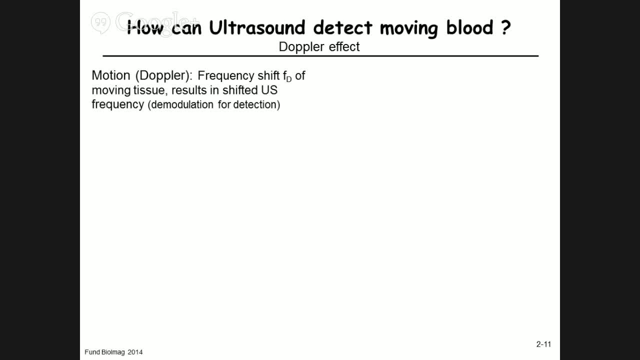 of the sound wave if the object is moving, In this case if there's moving tissue. This results in a shifted ultrasound frequency that can be detected with a demodulation. So that's just detecting a different sine wave, to make it simple. 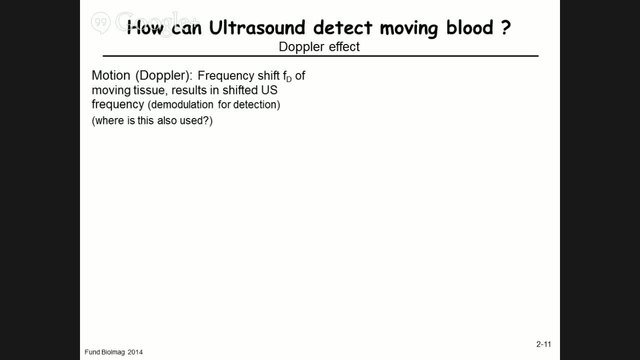 Okay. so where is this elsewhere used? I have shocking news for you. You have been exposed to the Doppler effect today. You just don't know. it probably Okay. How many of you have gone to Arkady? Pretty much everyone. 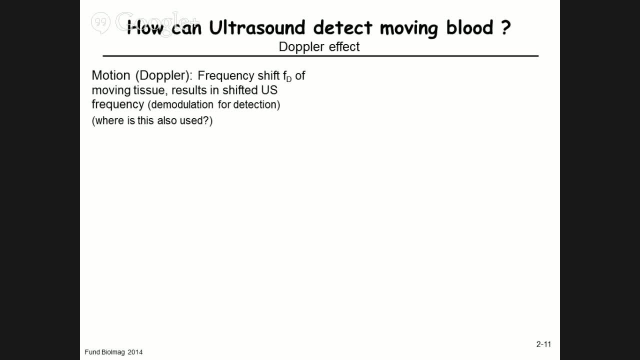 Come on, admit it. Or if you walk through CM and you go over to the cupol, you walk through some doors that open magically. Right Ever stood in front of the door and not moved. It, closes again and pretends like you're not there. 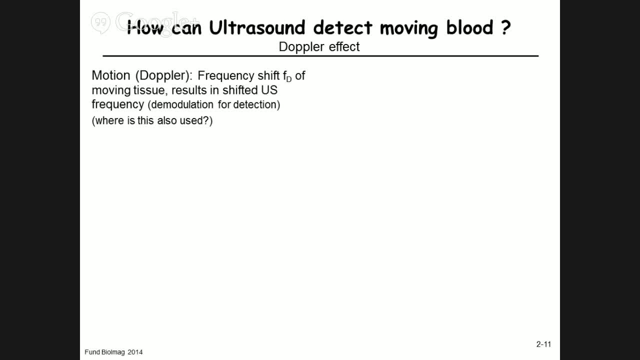 So what does the door do? What's in the door is an infrared diode that emits infrared light and when it gets back through the moving object, the wavelength of the light is slightly shifted through the Doppler effect and that interference is detected. 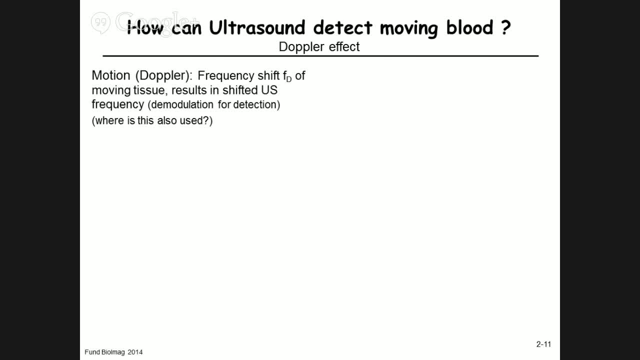 That's why, when you stand in front of the door and you don't move, it will close. When you move, it will open. That's how it detects motion, But it's a Doppler effect with electromagnetic waves. Okay, so if we look at sound, 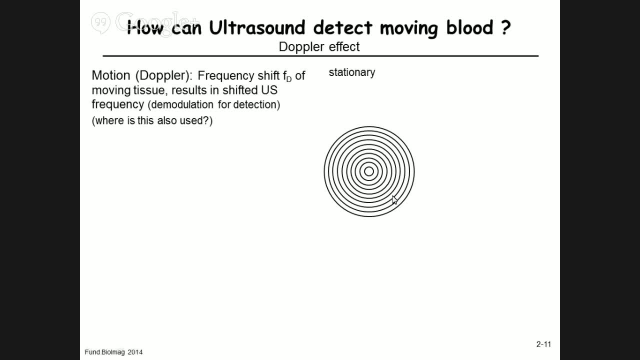 stationary, I produce a sound, it'll propagate with the same wavelength in all directions. If the source of the sound is now moving, it moves closer by V0t, to the observer here on this end. and so now the separation of the wave maxima. 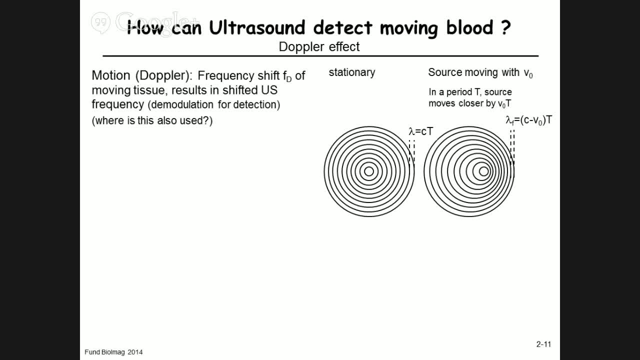 is now shortened by V0t. That gives you a change of apparent wavelength of C minus V0 times t in that period. t And here it's the opposite on the other side, because the object here is moving to the right, It's a prolongation. 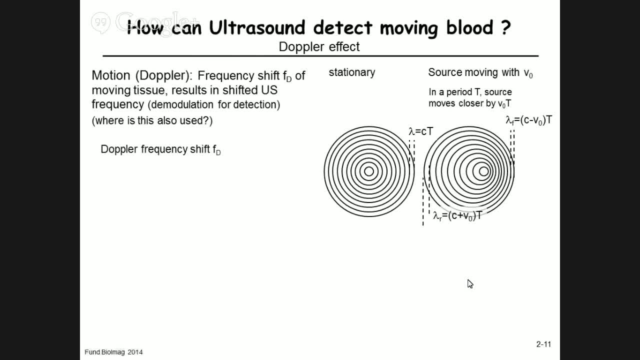 so it's an increase in wavelength. You have all heard the Doppler effect. Now this time, tell me you remember, Okay, Ever heard an ambulance or a police car approach you and then go away from you? Ever noticed a change in sound? 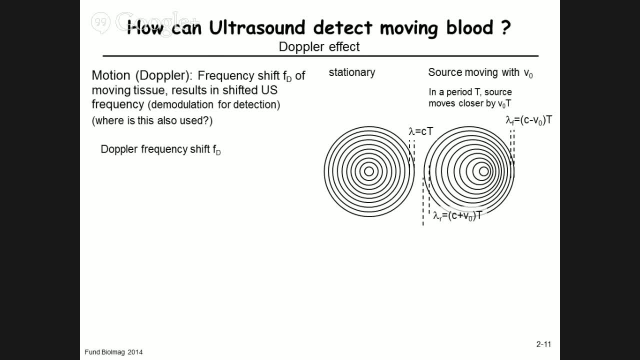 That's the Doppler effect. Okay, so the shift- and I'll just give you the empirical frequency without the demonstration where it comes from The Doppler shift- is two times the frequency, times the velocity of the object, times the cosine of the angle. 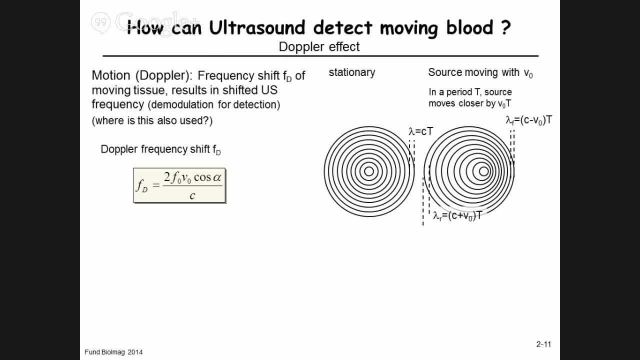 which is the angle of the observer relative to the motion divided by the wave propagation. velocity Doesn't really matter too much here. just to give you an idea, In tissue we have the speed of sound is one and a half kilometers per second. 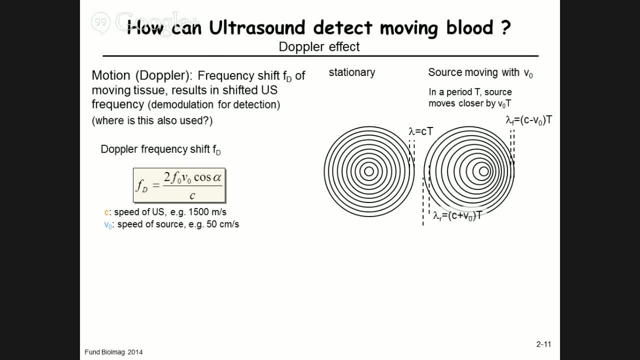 Let's say we take the speed of the source, that is, blood in an artery, about 50 centimeters per second, The frequency of the moving source. now, here we don't have a moving source, but we have a reflection in a moving source. 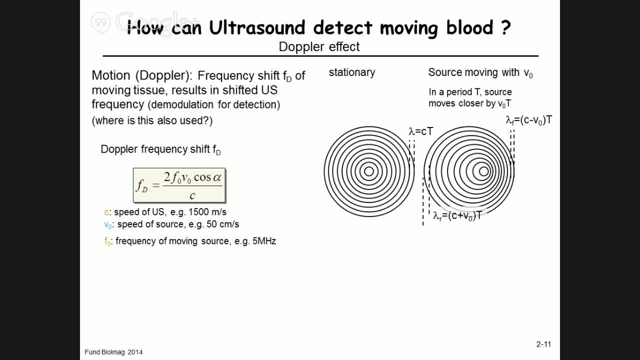 at an object that moves, That's the same thing as the source is moving, And so the frequency of the ultrasound is five megahertz. Okay, we've dealt with the angle here and now we can give an example. So if we take this example, 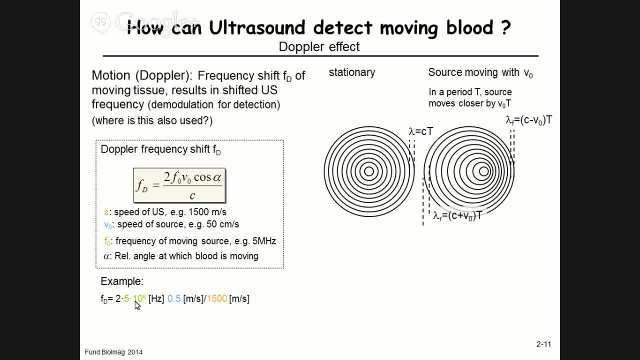 we've got five megahertz of frequency, we have got the factor two, we have the velocity, which is a half a meter per second, we have the wave propagation velocity and if you do that you get a shift in Doppler. 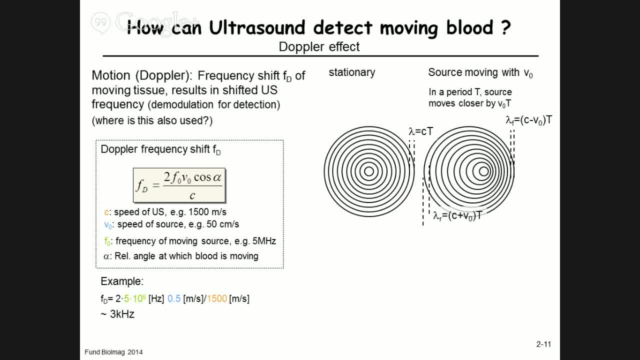 in ultrasound frequency of three kilohertz. Yay, that sounds wonderful. Three kilohertz, that's not bad, huh? Well, it's .05% of the ultrasound frequency, So it's a small shift, but the good thing is about electronics. 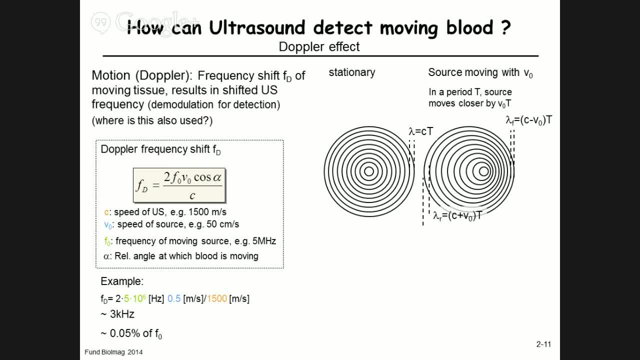 and today's detectors. a three kilohertz shift with demodulation is easily measurable with the appropriate electronics. So what you observe is the Doppler shift here. that is then decoded the frequency shift, because you demodulate the frequency. 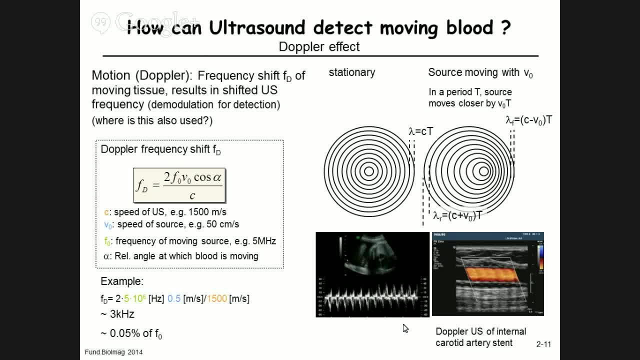 and you can see the moving blood. So this is now an example of an internal carotid artery stent. so it's a reinforcement for somebody who has some vascular problems. and if you look at it now, in red is the Doppler demodulation. 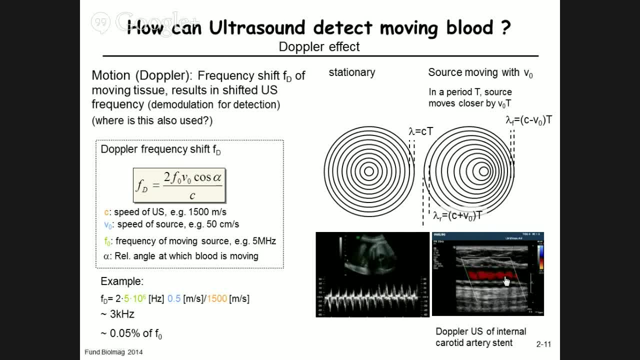 behind is the static ultrasound image that you can still reconstruct, and now you see the pulsatile flow of blood and, because the stent has some cylindrical structure with reinforcements, at a certain distance you can see the turbulences of the blood flow. in this case, 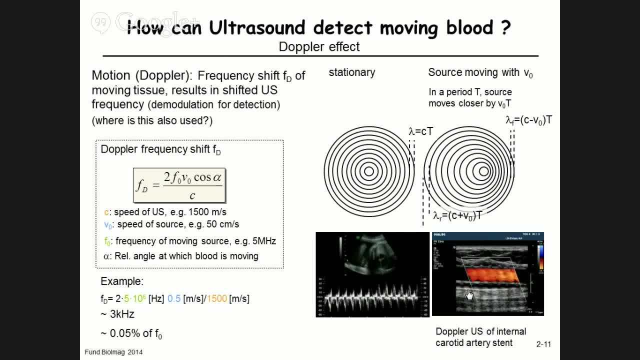 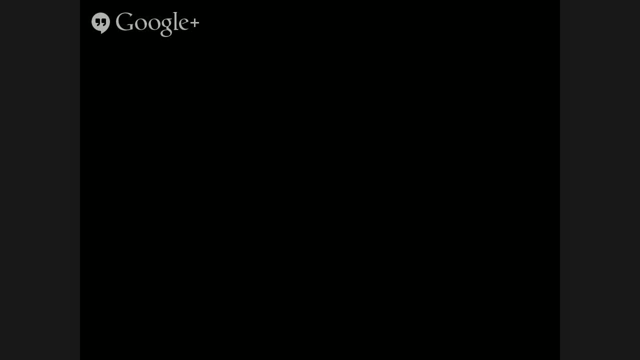 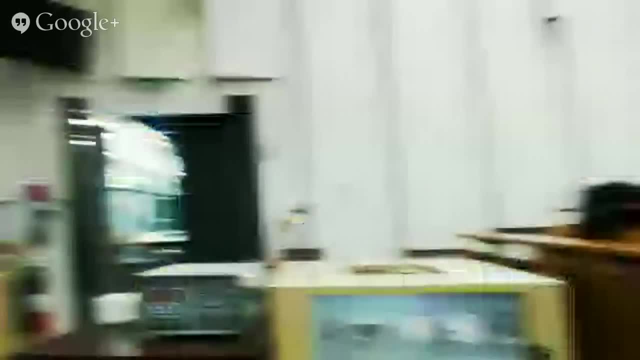 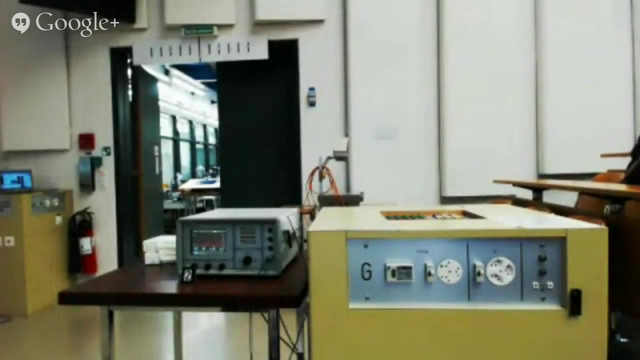 Somebody's talking here on the video, So just before the break I am going to try to demonstrate the Doppler effect here. So what you have on. actually, the better way is to show you the camera output as well, so I can show you. 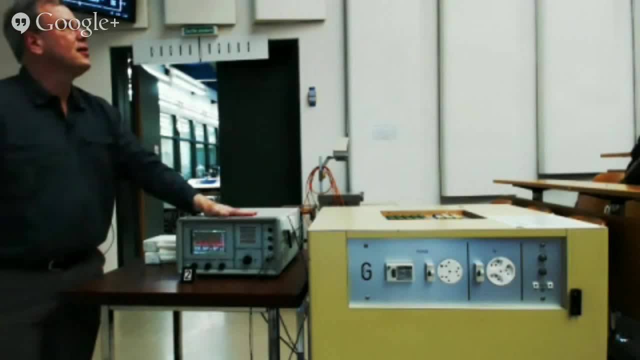 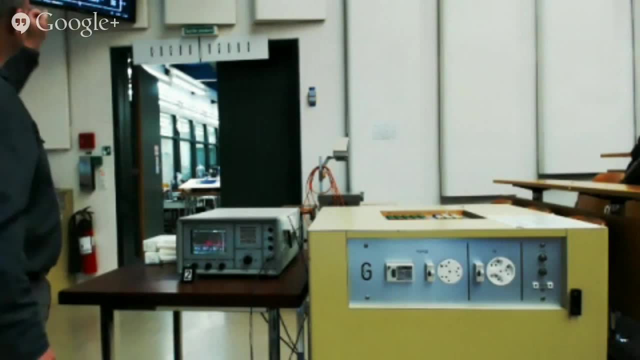 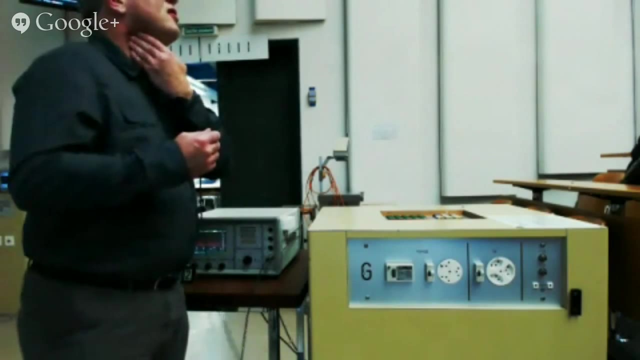 you have it on the screen overhead. this is an ancient ultrasound detector- Doppler ultrasound from the labs here. what you have on the screen is the signal that it detects. what I am now going to do is see if I can see my 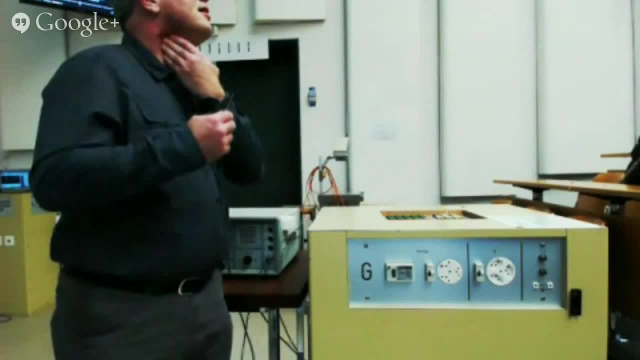 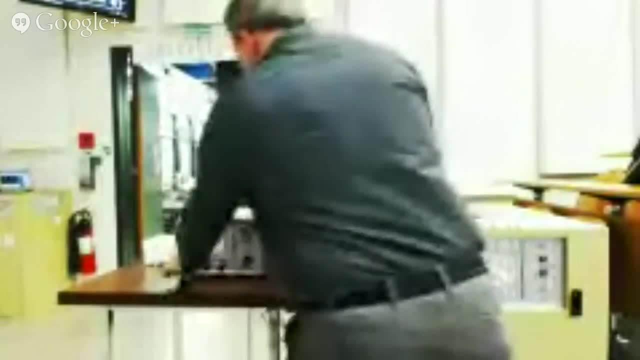 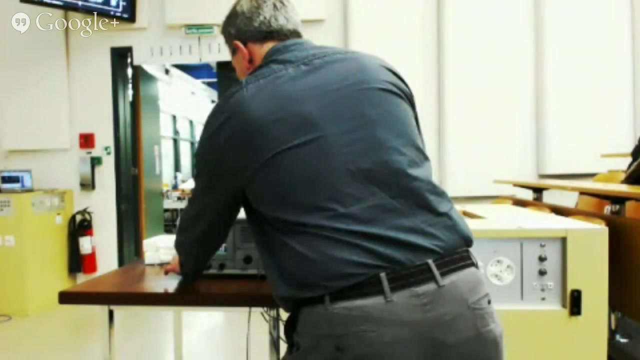 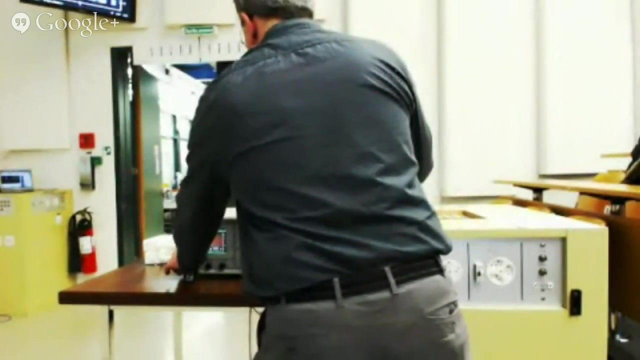 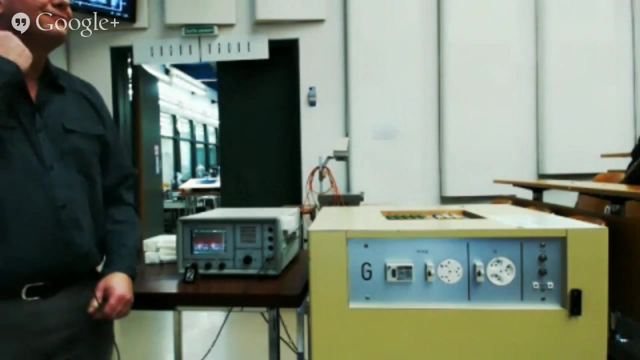 jugular artery, the pulsation on it. Can you hear it Right? It's very fast. That's the nervosity of the teacher. but this is what you also hear when you observe a baby in the fetus. it goes all the.